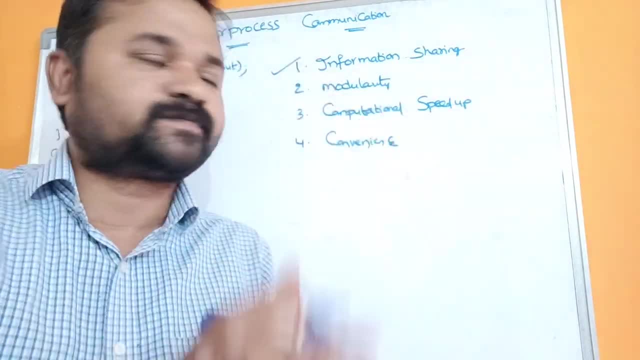 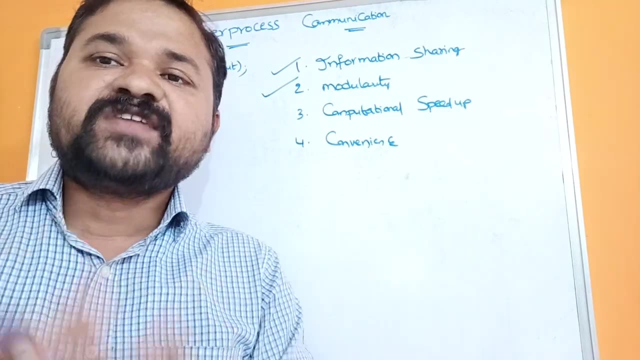 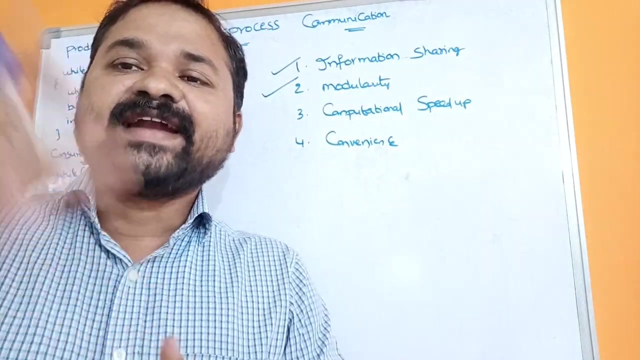 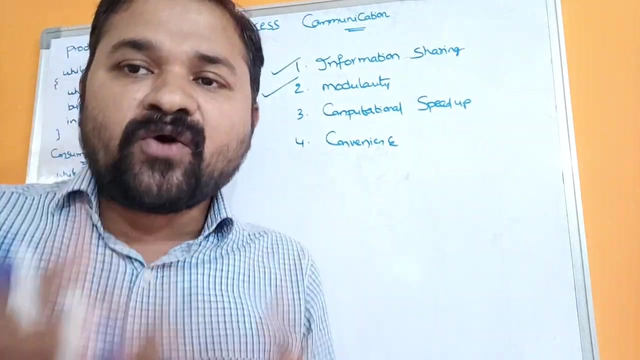 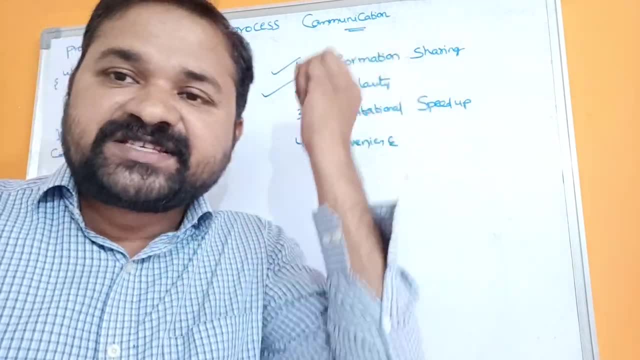 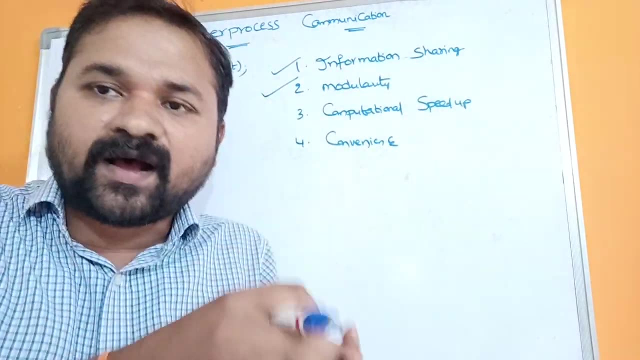 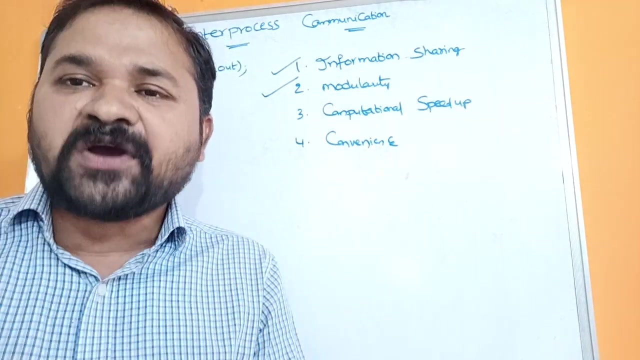 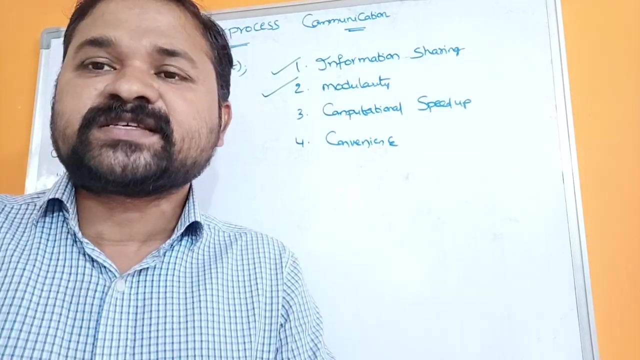 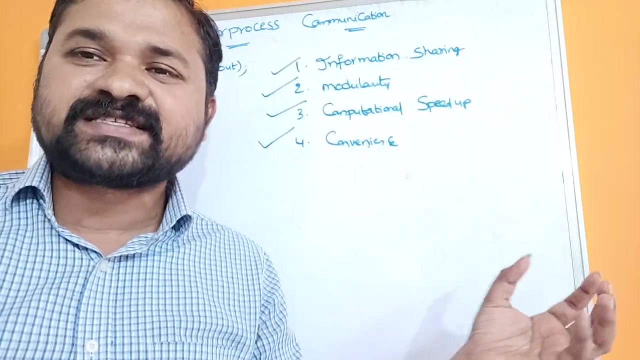 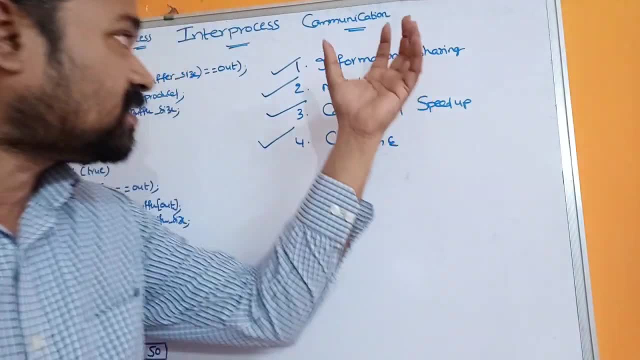 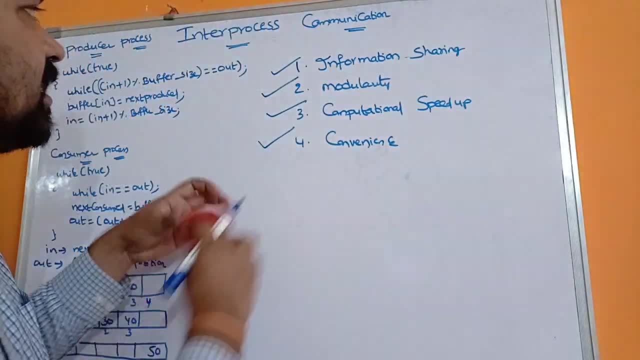 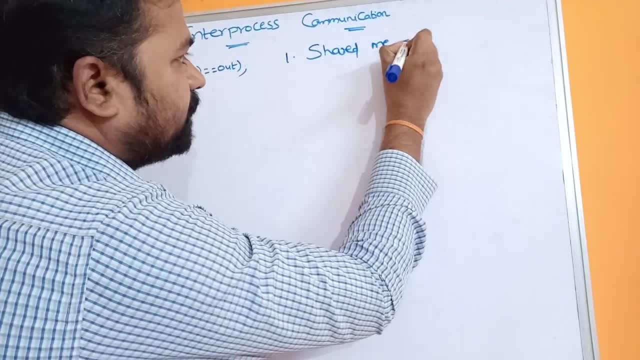 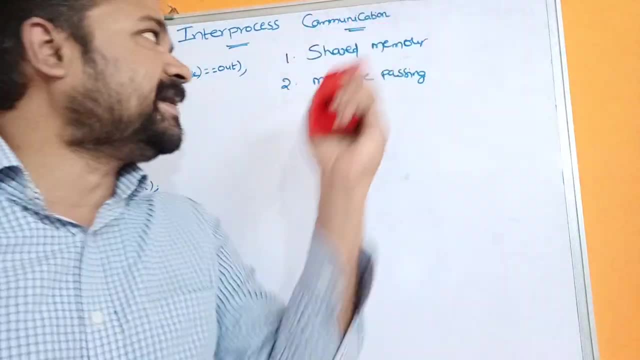 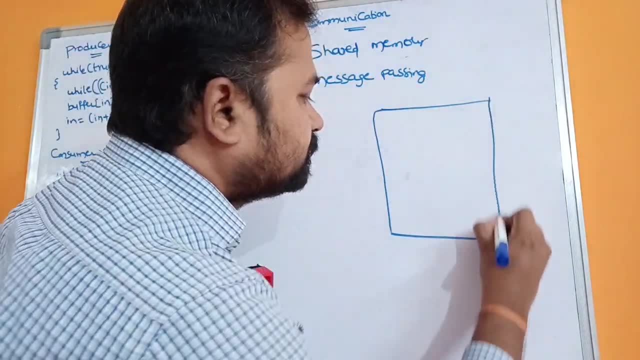 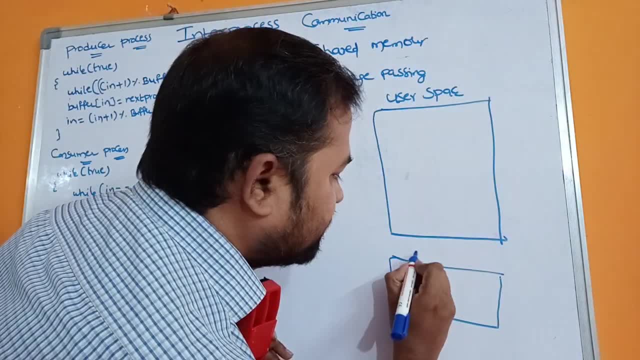 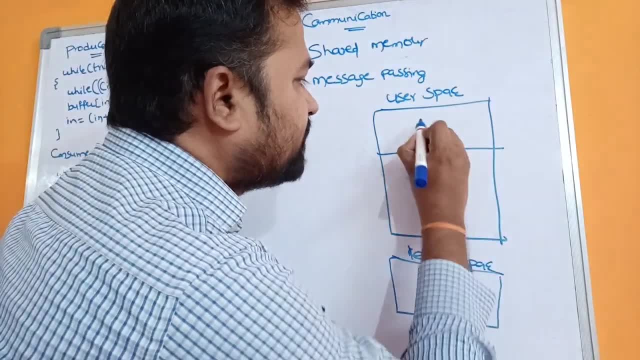 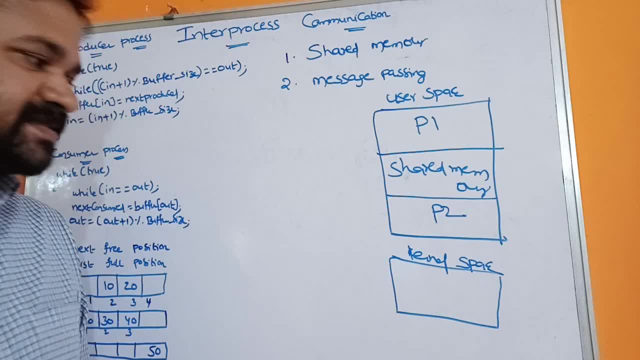 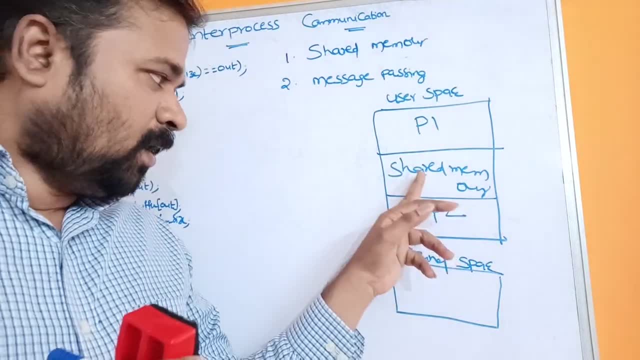 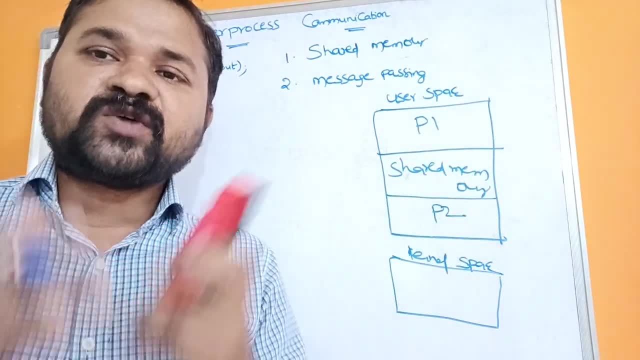 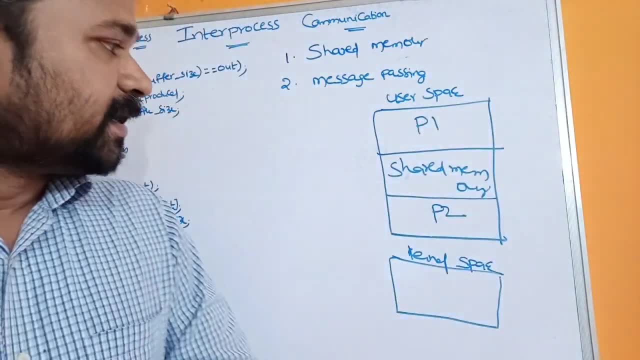 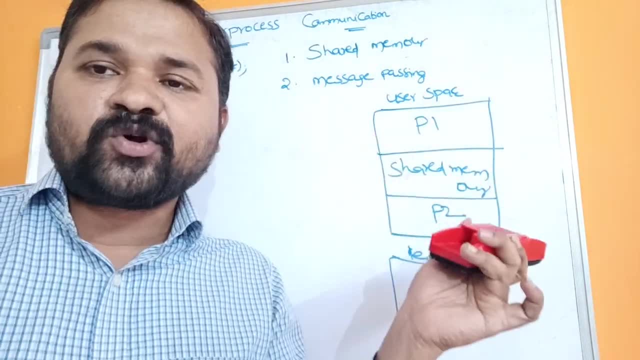 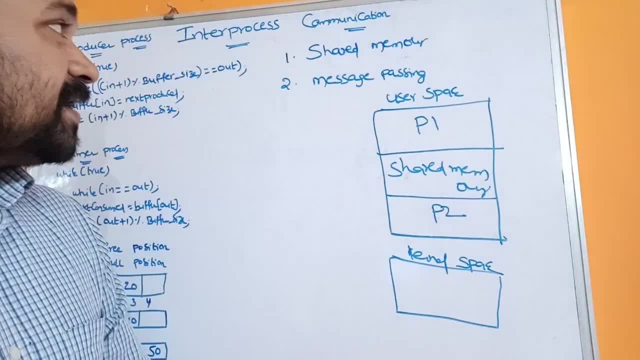 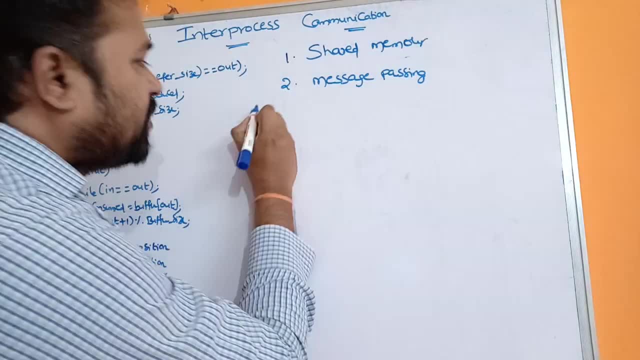 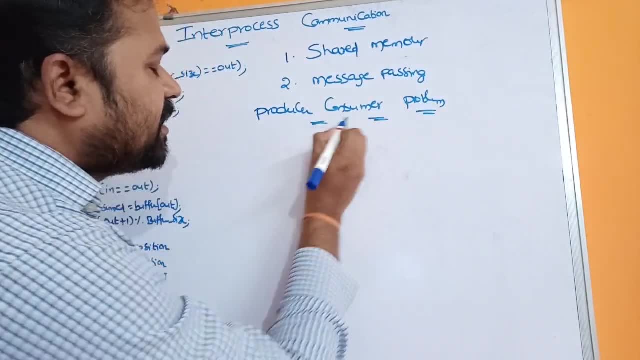 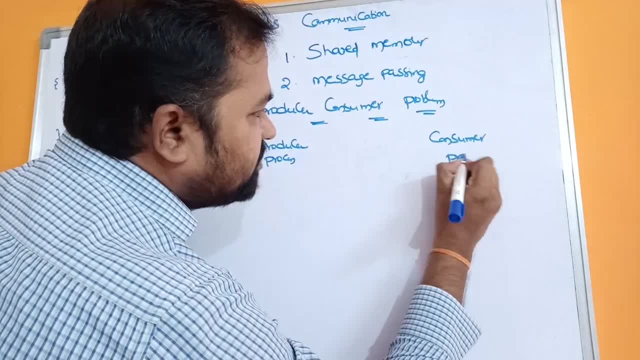 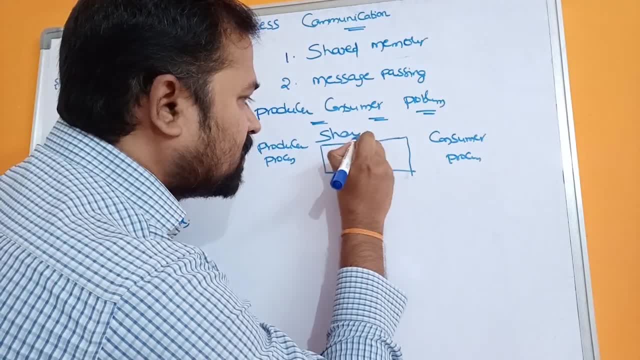 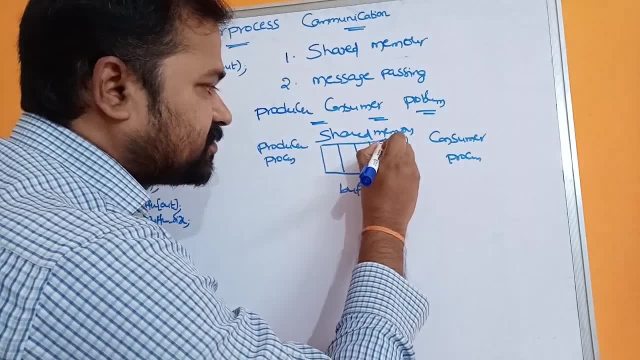 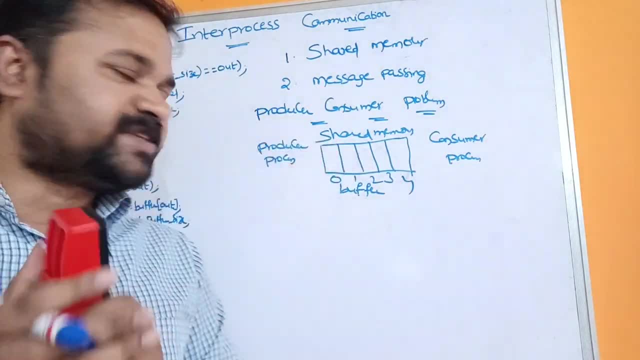 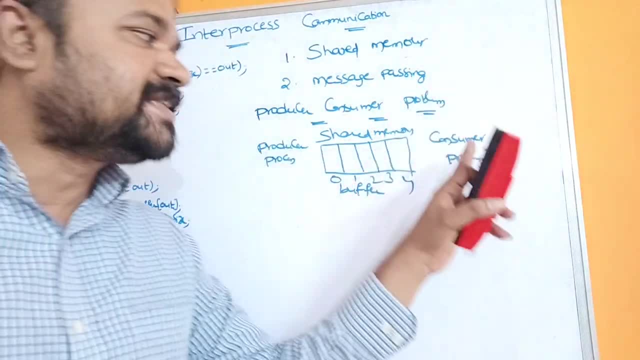 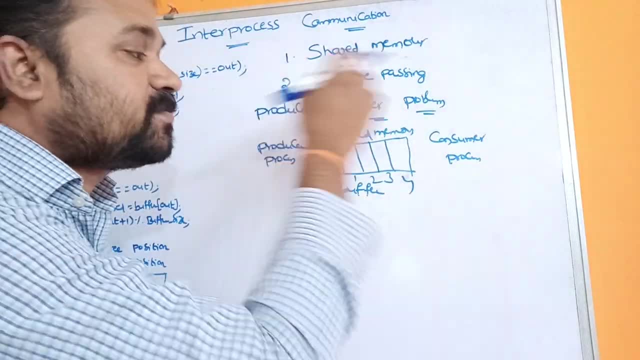 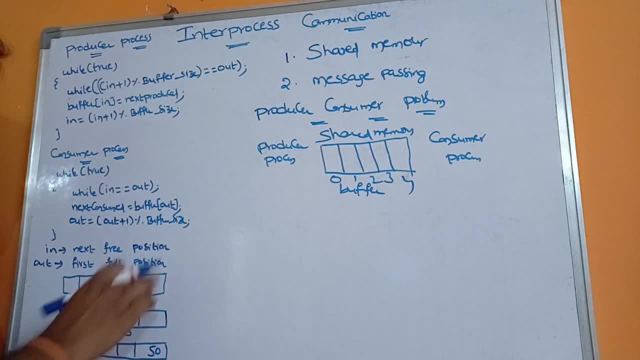 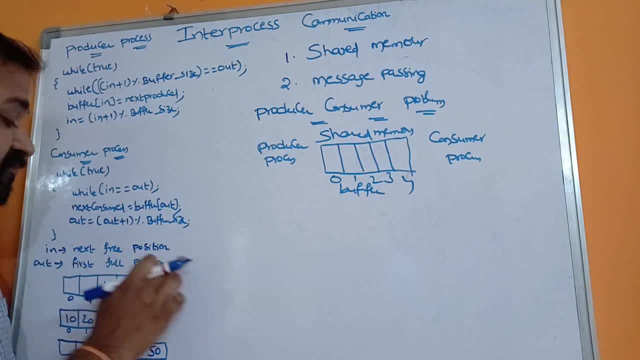 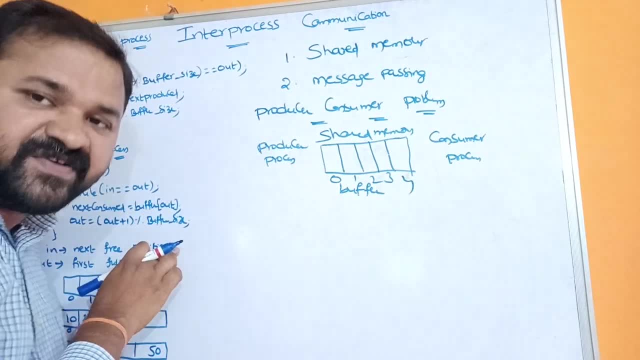 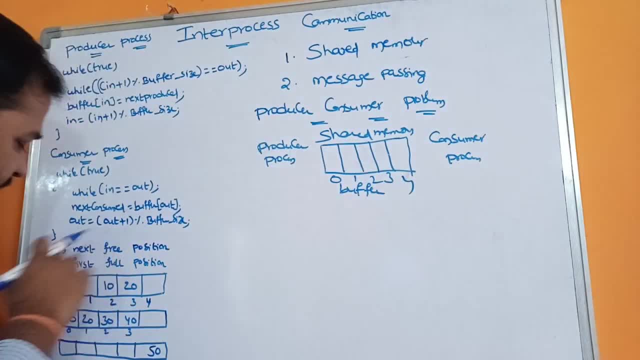 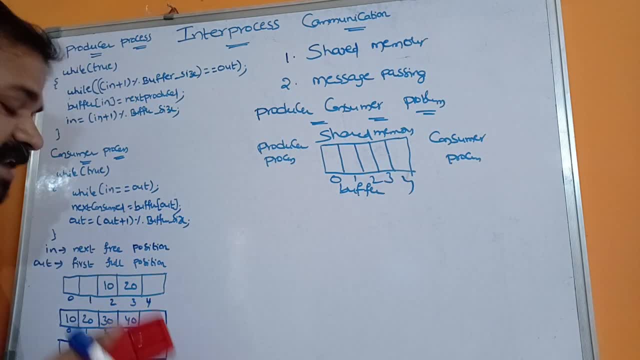 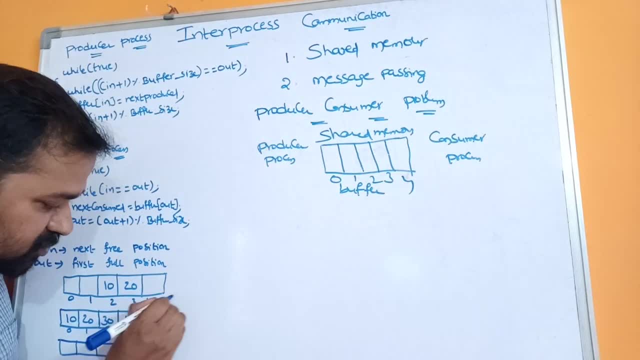 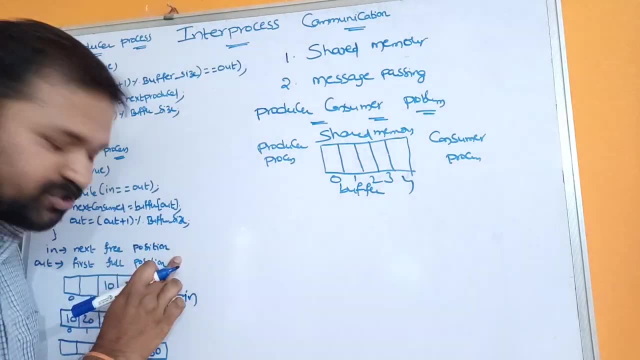 So what is the next free position? 4 is the next free position. So this 4 is nothing but in, Whereas what is out Out always points to the first free position. Here we have two items. The first item resides at second position. 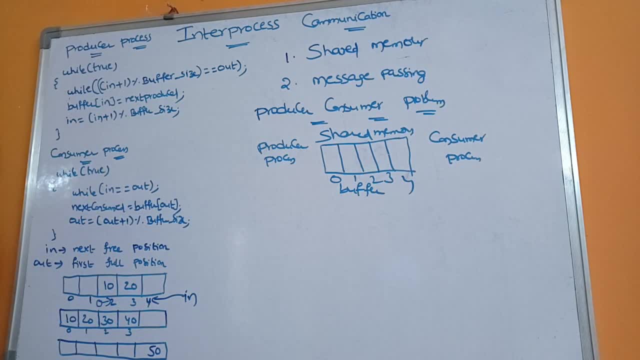 So this 2 is nothing but out. Okay, Now let us consider the code for producer process Here. while of true true means this condition is always true. Let us observe about this condition later. First, let us see the code here. 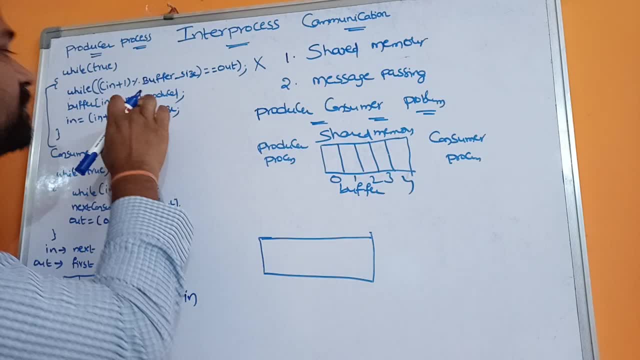 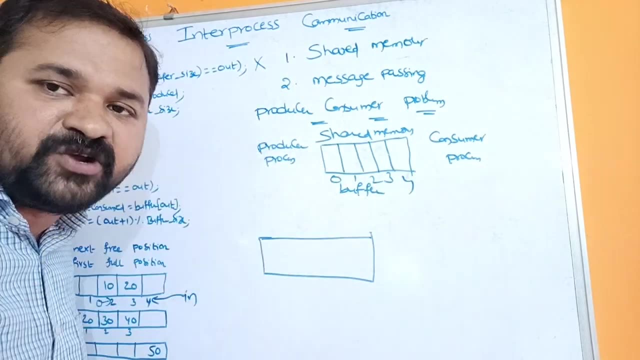 Producer process produces an item And that item will be stored in a variable called next to producer. So next to producer is nothing but an integer variable. So producer process produces an item And the corresponding item is stored in a variable called next to producer. 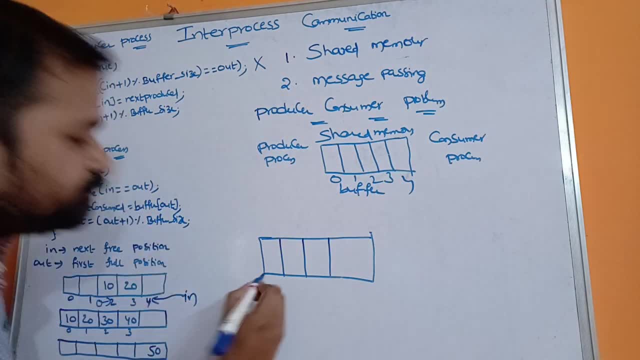 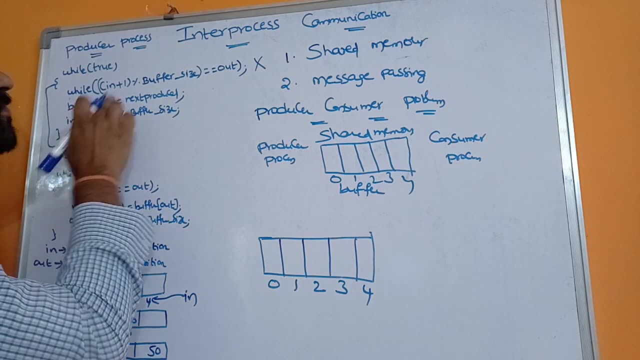 Let producer process produces an item And that item is called 10.. So 0,, 1,, 2,, 3,, 4. So 10.. So next buffer of in is equal to 10.. The initial value of the in and out is 0.. 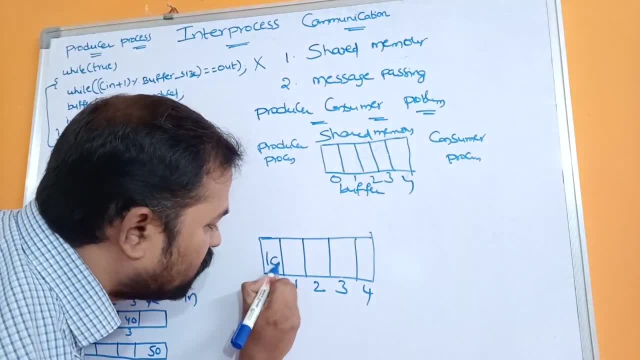 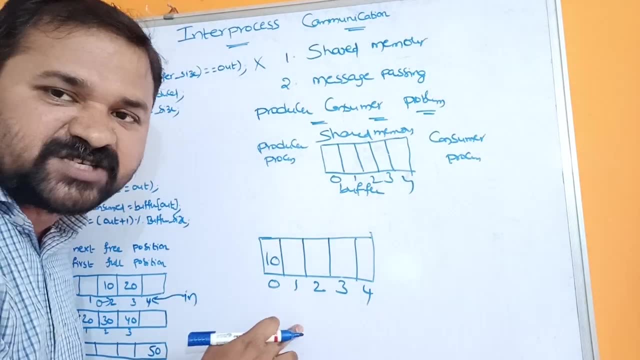 So buffer of 0 is equal to 10.. So 10 will be stored in 0th location. Next, in is equal to in plus 1 modular buffer size, What is in value 0. So 0 plus 1 means 1.. 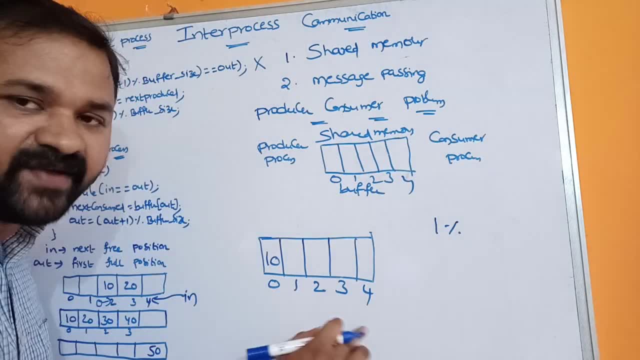 1 modular buffer size Here. what is the buffer size? 5. 5 is the buffer size, So we can have, We can have items from 0 to 4.. So 1 modular 5 means what? 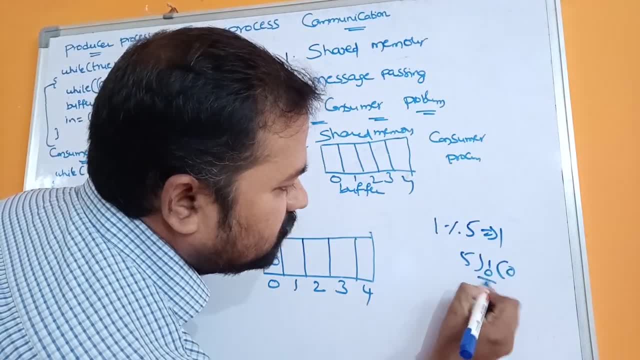 1. Okay, So 5, 1.. 5, 0, 0.. So this is nothing but remainder 1. So now, what is in value 1. So once again, control goes to the value. 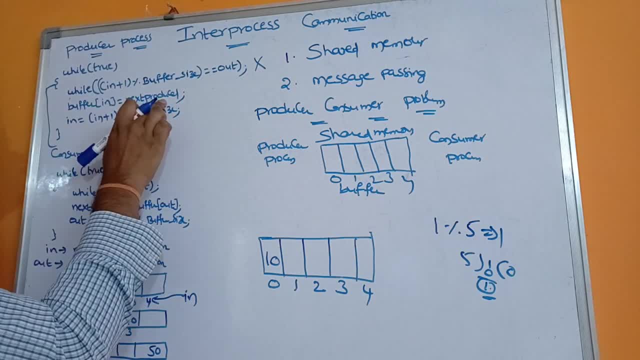 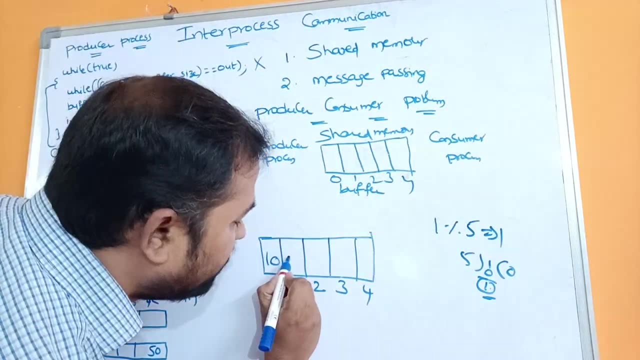 While after condition is true, Next buffer of in is equal to next to producer. So what is in value now 1.. So buffer of 1 is equal to next to producer. Let us assume that producer process produces an item called 20.. 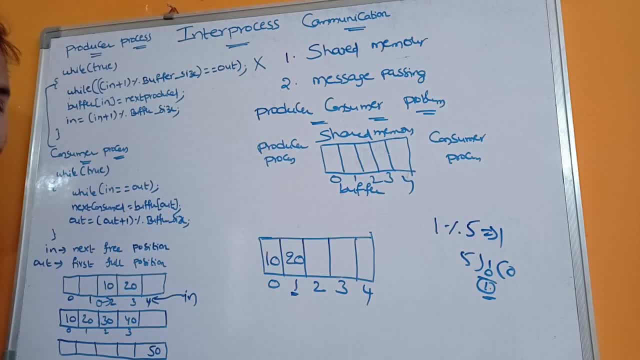 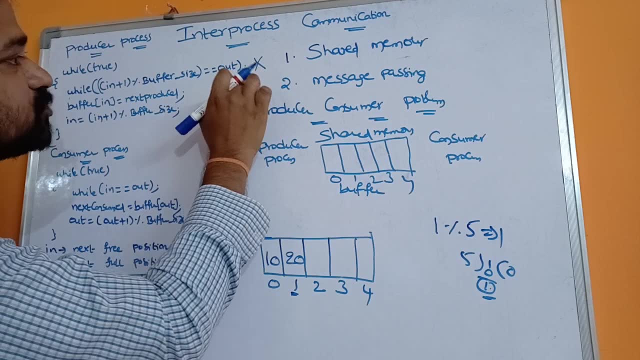 So 20 will be stored here. So, likewise, each time in will be incremented. Now let us see about This condition: While in plus 1 modular buffer size double is equal to out, While in plus 1 modular buffer size double is equal to out. 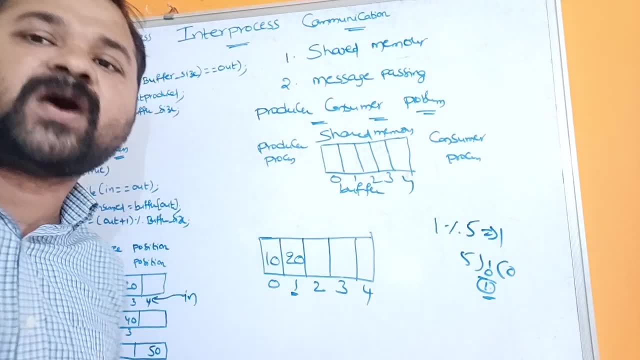 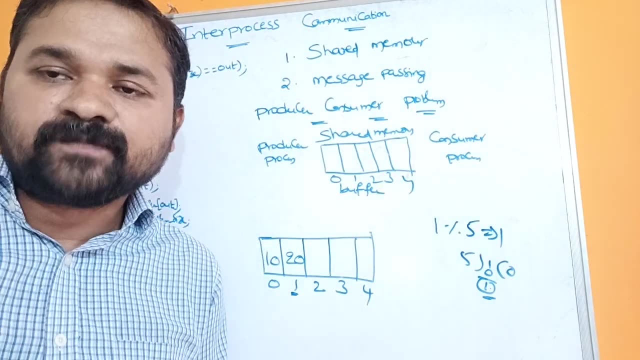 So whenever this condition is true, then we can say that the buffer is full. So first we have to check whether the buffer is full or not. If the buffer is full, then it is not possible to insert an item into the buffer. 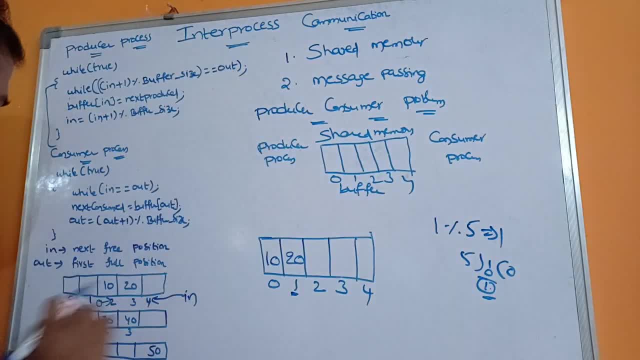 So first we have to check for that condition. Let us observe this work. Here we have. Let us observe this condition: Here we have 4 items, So 10, 20, 30, 40. Let us perform producer operation one more time. 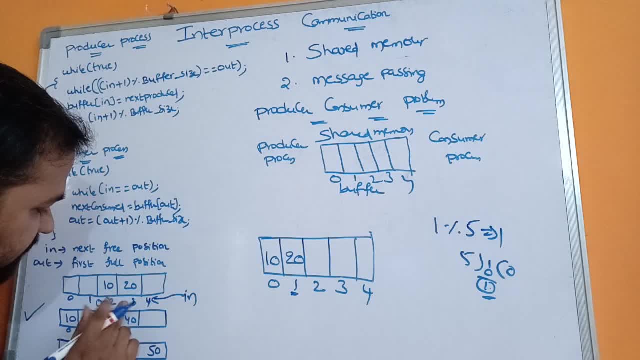 So what will happen? In plus 1. What is in value? What is in value Here? the value of in is 3.. So 3 plus 1 means 4.. So 4 modulo 5 means 4.. 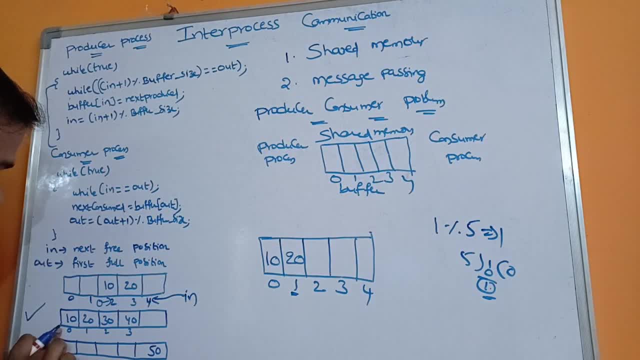 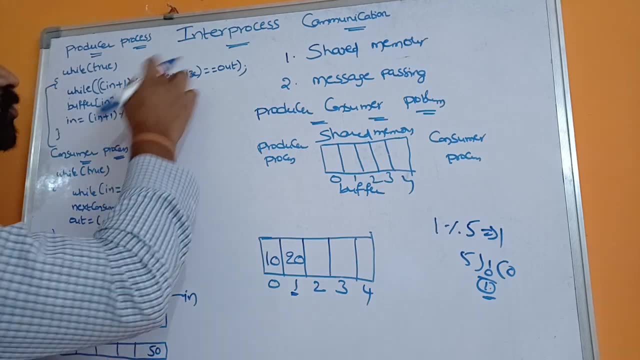 4 double is equal to What is out here. Out always points to the first full position. What is out here? In this example? here the first item is 10.. So out means 0. So the condition is false. 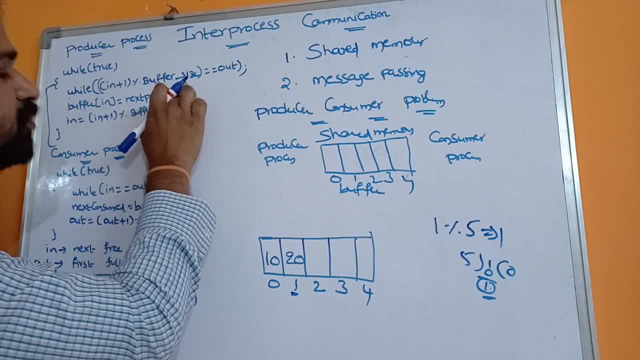 What is in? 3 plus 1 means 4.. 4 modulo 5.. I am sorry, What is 4 modulo 5?? Yeah, correct, only So 5: 0s are 0.. 4 minus 0 means 4.. 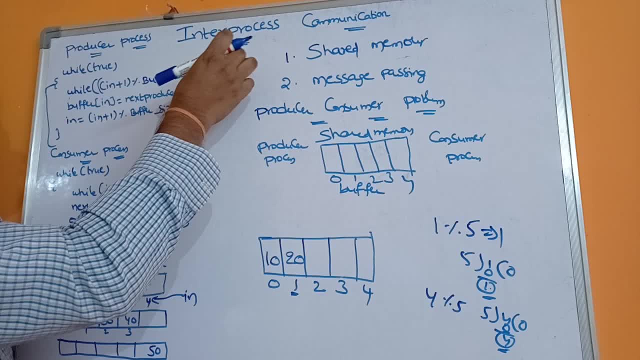 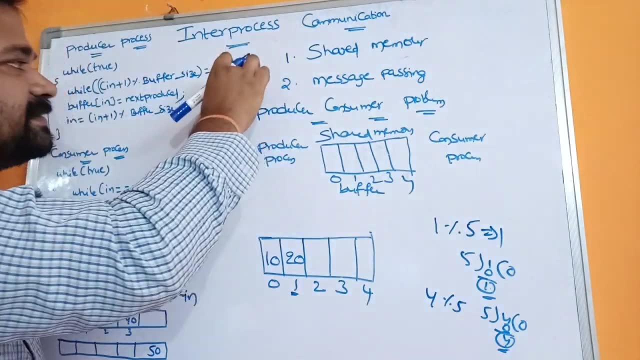 So 4 double is equal to 0. Condition is false, So that the control comes out from the while loop. Here we have semicolon. Semicolon means if the condition is true, then it remains in the while loop. 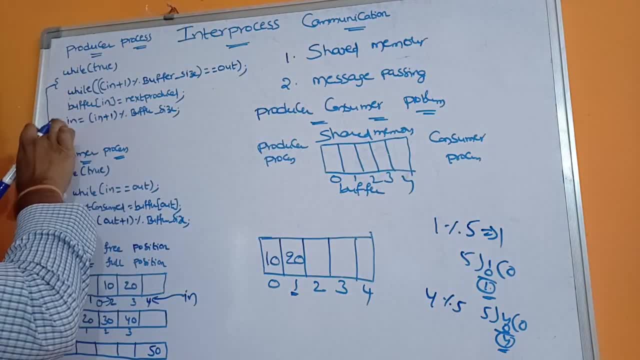 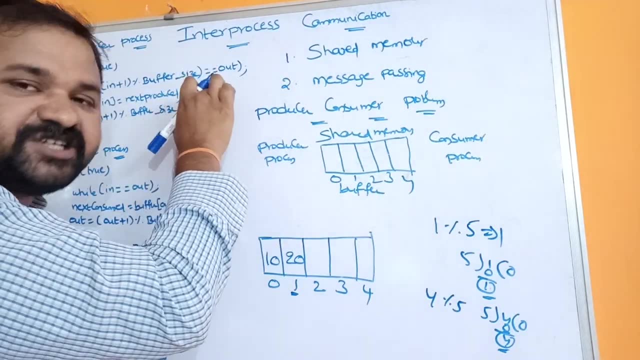 Whereas if the condition is false, then the control comes out from the while loop. Here we have. These two statements are not belonging to the while loop. These two statements are separate statements. So if the condition is true, then the control remains in the while loop. 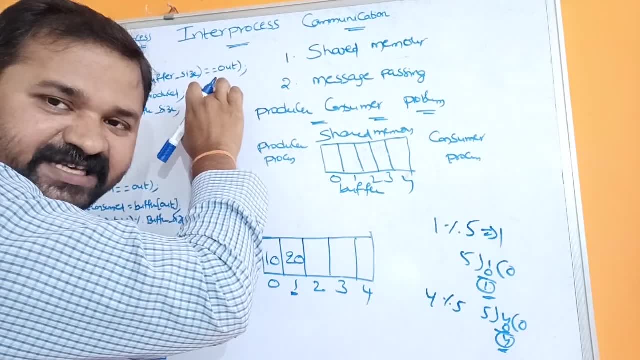 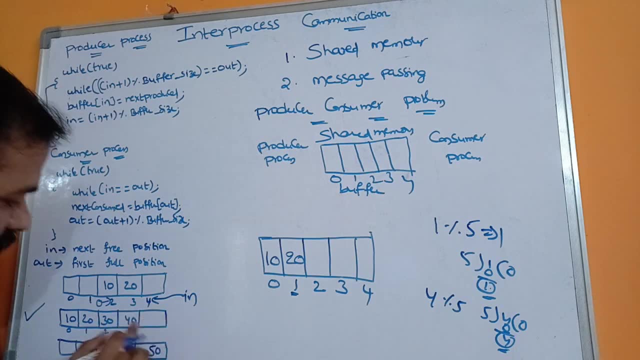 Okay, That is nothing but some infinite loop. If the condition is false, then only the control comes out from the while loop. So buffer of in is equal to next produced. So what is in now? What is in The value of the in is 4.. 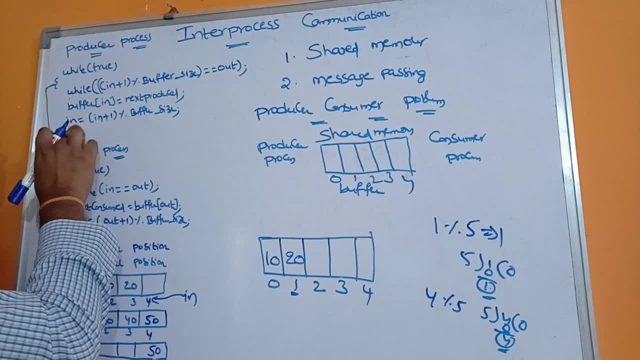 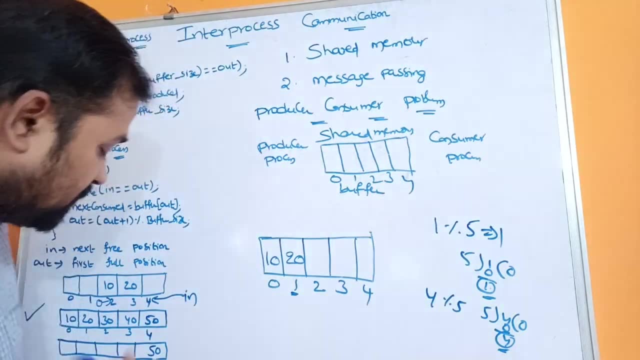 Okay, So 50 will be inserted here. Okay, Next, in is equal to in plus 1 modulo buffer size. In is equal to In plus 1 modulo buffer size. So what is the previous value in Here? the previous value of in is 3.. 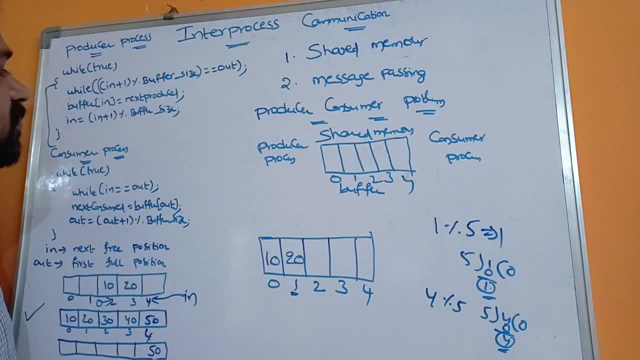 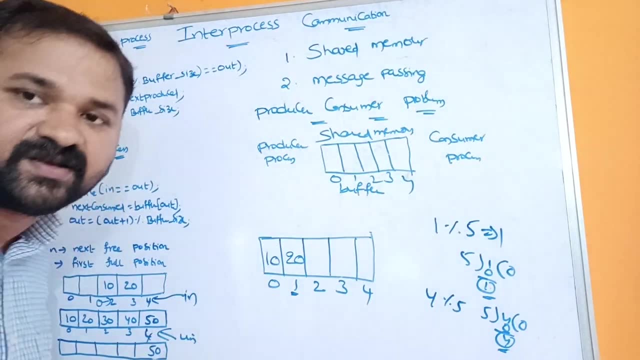 So now, 3 plus 1 means 4.. 4 modulo buffer size means what? So what is the This 4.. Okay, Now this in will be at the 4th location. So now what is out? 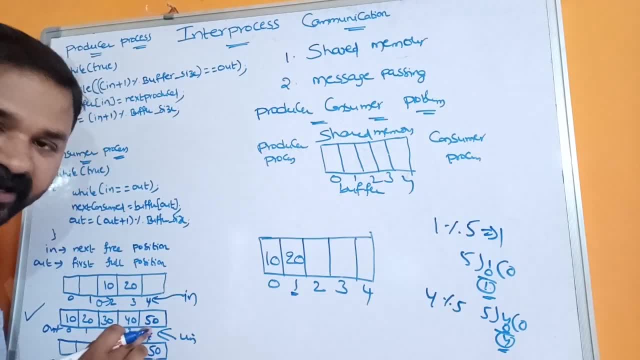 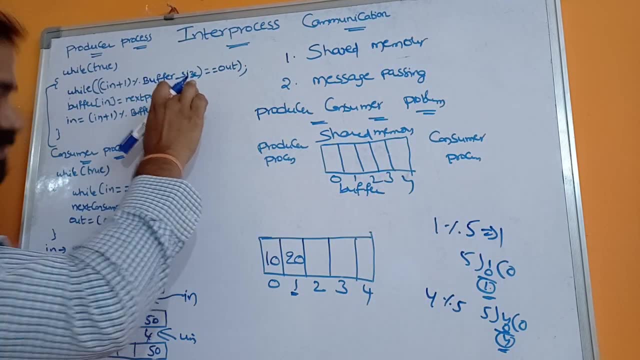 Out is at 0th location, Whereas in is at 4th location. Now the buffer is full. Let us check whether our program is correct or not. Why in plus 1 modulo buffer size, What is in 4.? 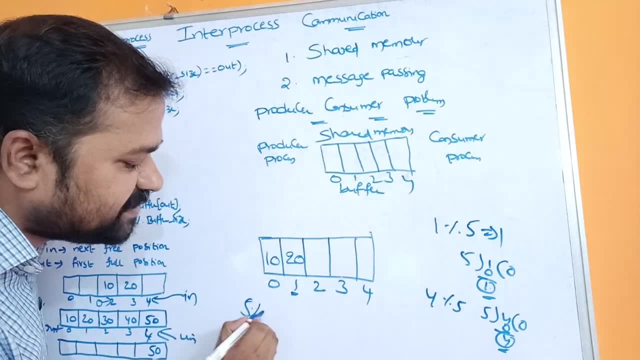 4 plus 1 means 5.. 5 modulo 5 means What is 5 modulo 5? 0.. So 0.. If we give 0 as the result, 0 double is equal to what is out. 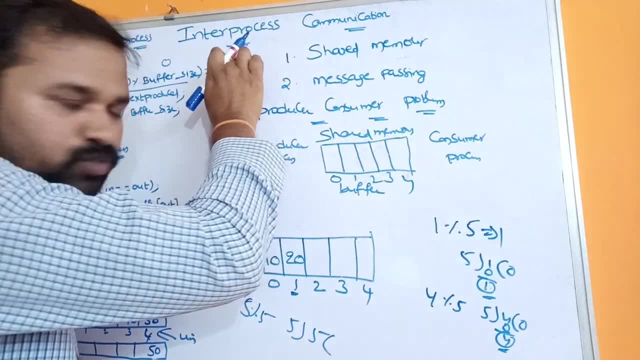 Out means 0. So 0 double is equal to 0.. Condition is true: Here we have semicolon. If there is a semicolon at the end of the value, then the control stays in this loop only. Okay. 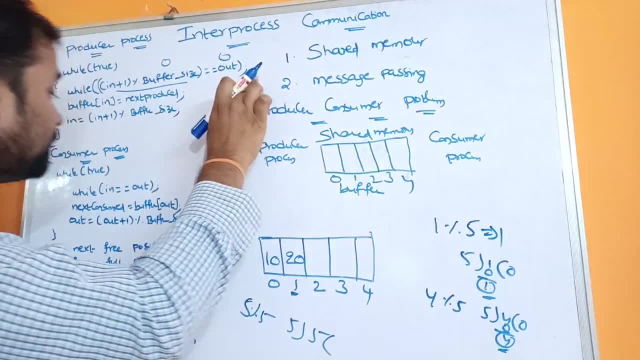 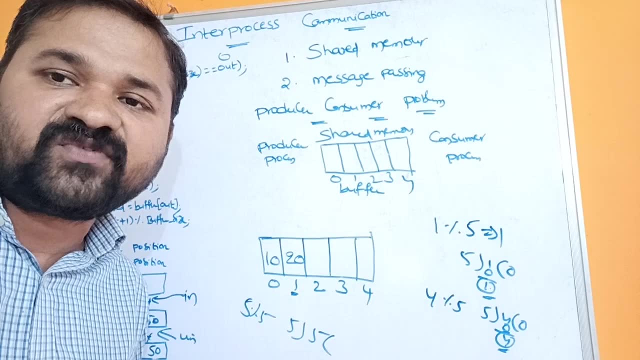 So this is the condition for whether the buffer is full or not. Now let us check for the consumer process. Okay, So before the consumer is consuming an item from the buffer. So first we have to check whether that buffer is empty or not. 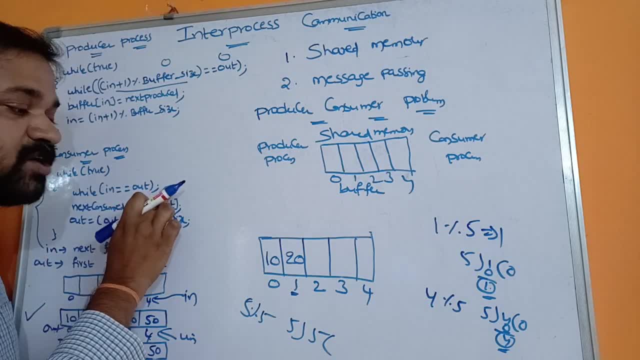 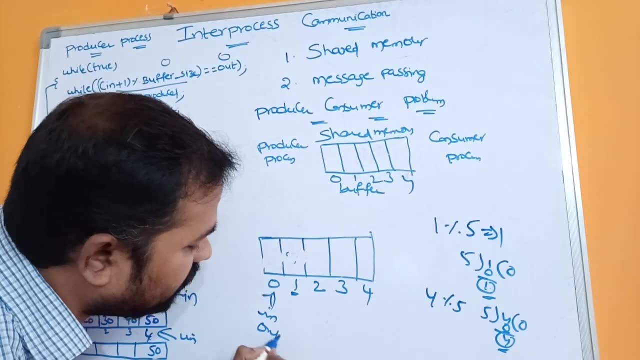 When we can say that the buffer is empty? Why? in double is equal to out semicolon. Let us assume that in and out are at the same location: 0, 0.. Okay, So what is in 0.. 0 double is equal to 0. 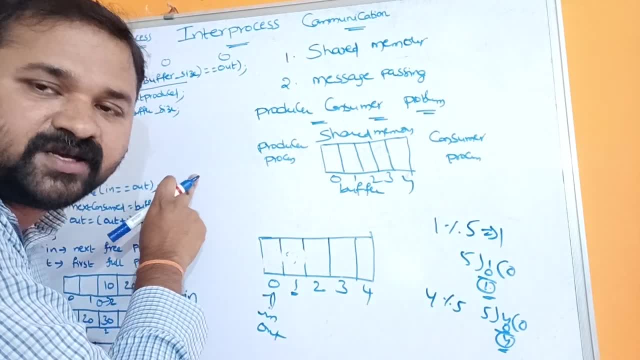 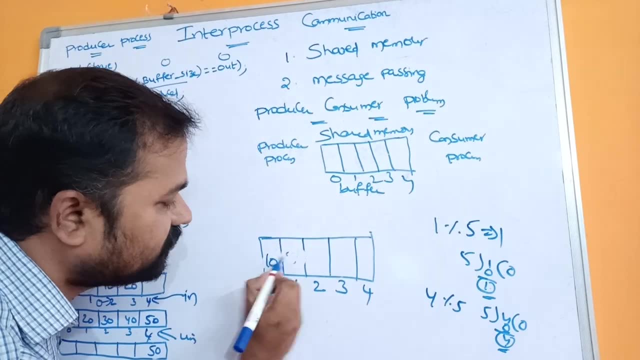 Condition is true. Semicolon, That means the buffer is empty. Okay, So the consumer has to wait until the producer produces some item from the buffer. Okay, Let us assume that We have three items here, So 10,, 20, 30. 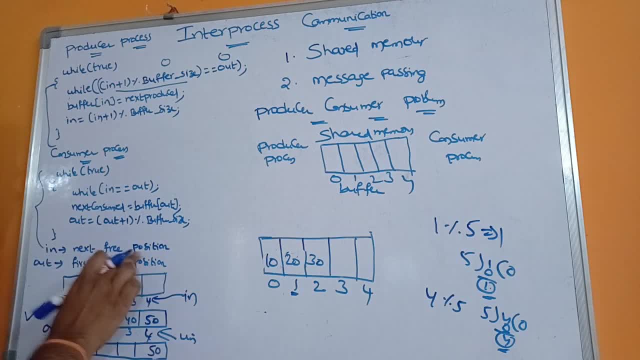 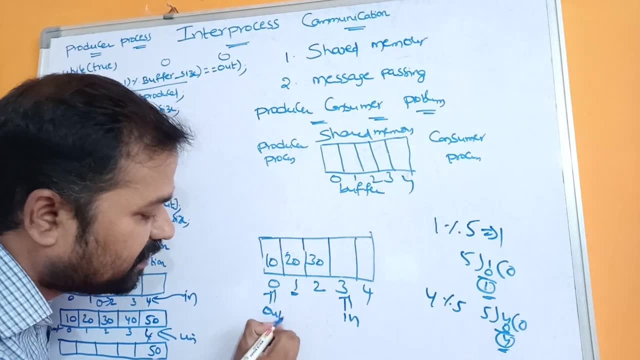 10,, 20, 30. So what is in and what is out. What is in: In means next free position. What is the next free position? 3. What is out- Out means first full position. Let us perform some consumer operations here. 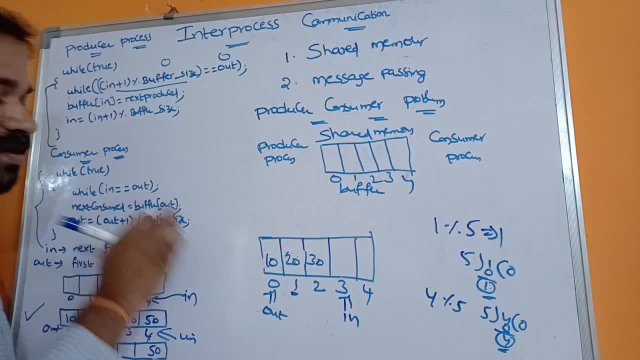 Okay, So what is the code here? Why in double is equal to out What is in 3. What is out? 0. 0 double is equal to 3. False, So control comes out from the while loop. 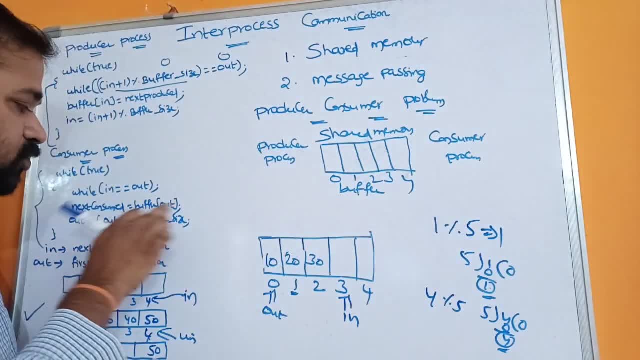 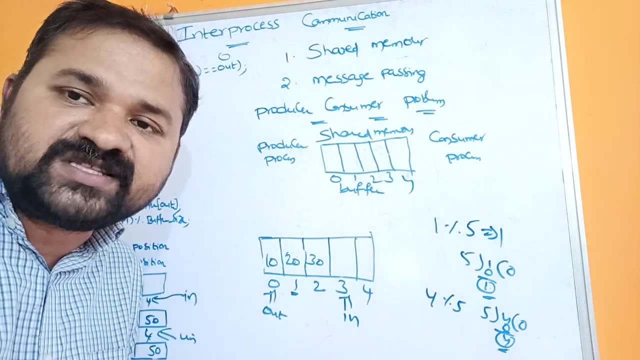 Here we are using a variable called next consumer. So buffer next consumer is equal to buffer of out. We know that consumer process consumes an item from the buffer and stores that item in a variable called next consumer. So what is buffer of out? 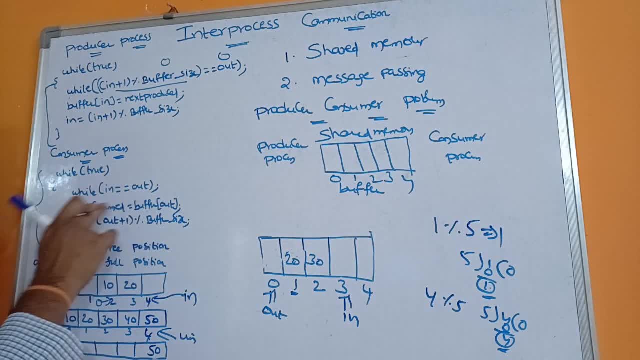 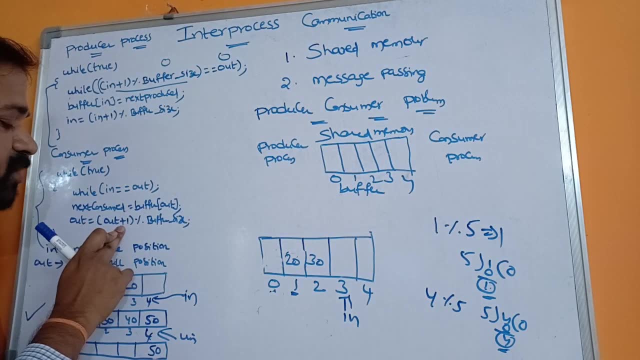 Buffer of 0.. So buffer of 0 will be consumed and it will be stored in next consumer variable. Okay, Next. So this 0 will be deleted. Okay, 0. item Next out is equal to out plus 1 module of buffer size. 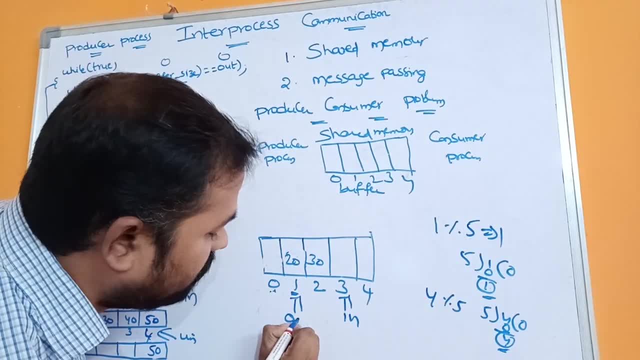 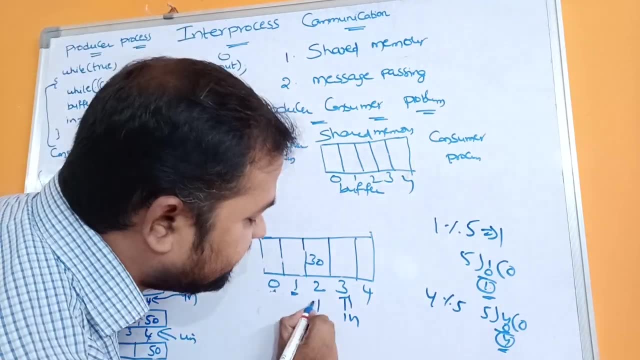 So 0 plus 1 means what? 1.. So 1 module of buffer size, 1 module of 5 means 1.. Next, what will happen? 20 will be consumed and out will be placed at this location. 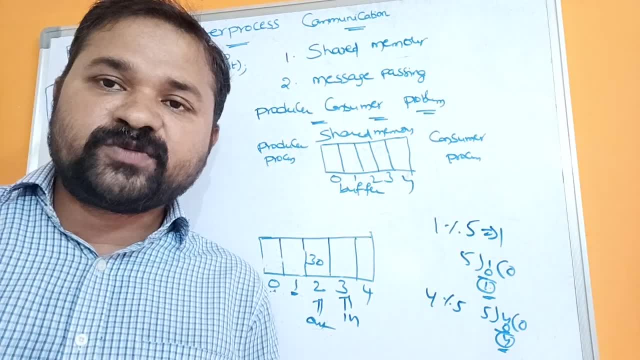 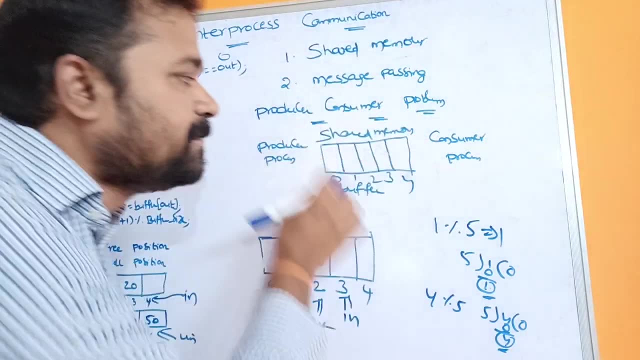 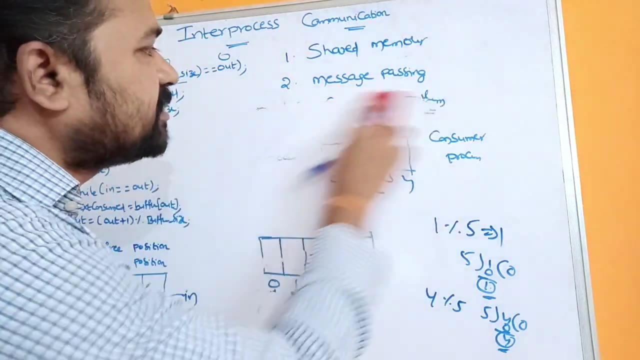 So this is about producer-consumer problem. So producer-consumer problem is the best example for this shared memory. So here we are implementing, Here we are using the shared memory in order to implement producer-consumer problem. So this is about producer-consumer problem and this is about shared memory. 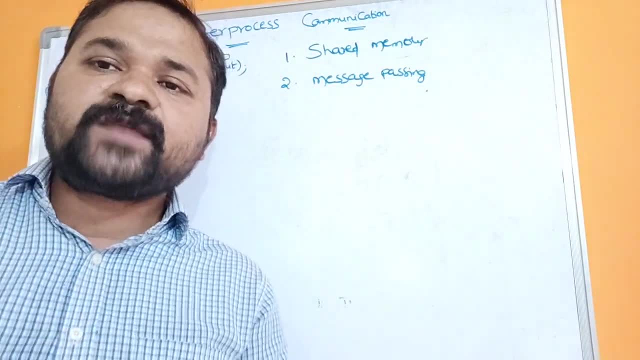 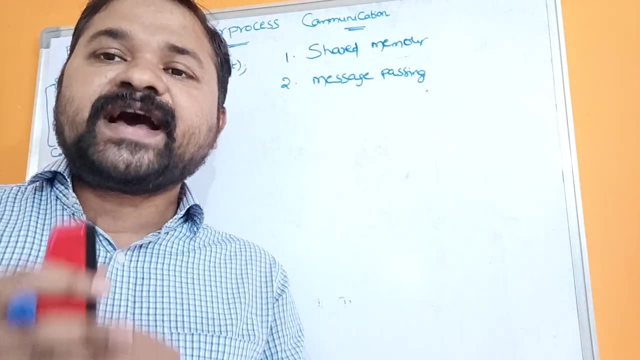 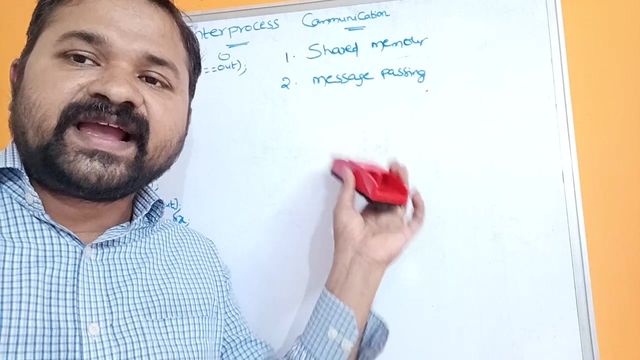 Now let us see about message passing In shared memory. producer process can communicate with consumer process with the help of a shared memory, Whereas in consumer process, whereas in this technique message passing, one process can communicate with other process with the help of messages. 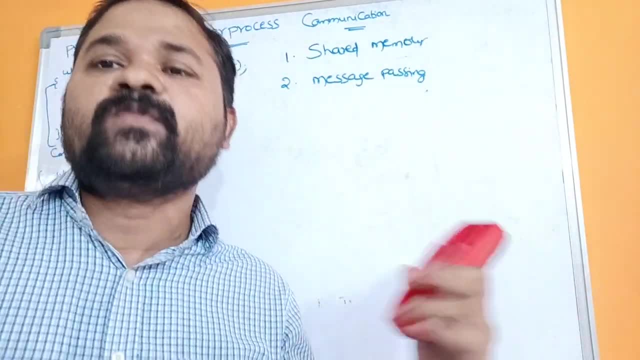 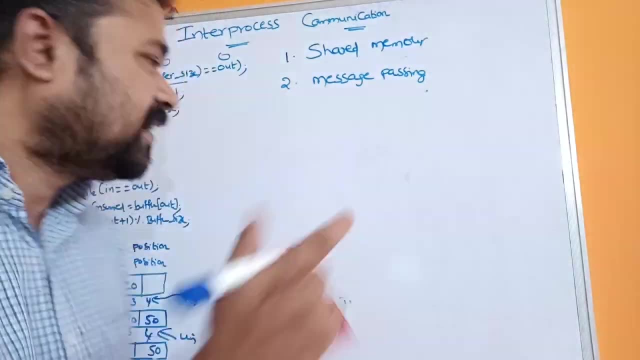 So message passing means here we did not use any shared memory concept, So one process can communicate with other process with the help of some messages. Okay, Let us take the diagram here. So let me have a. let me have a user space. 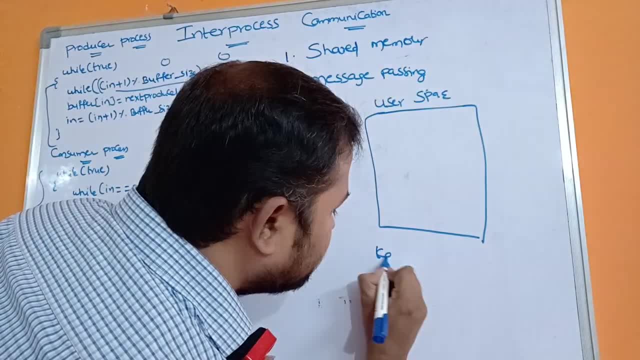 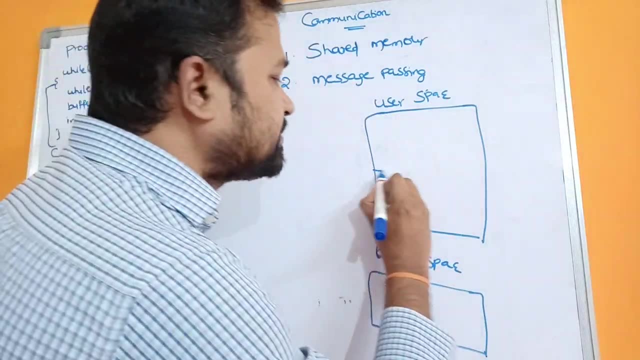 This is main memory, So main memory is divided into two parts. The first two part is user space, Whereas the second part is kernel space. Okay, So user space contains some processes. Let me have two processes: P1 and P2.. 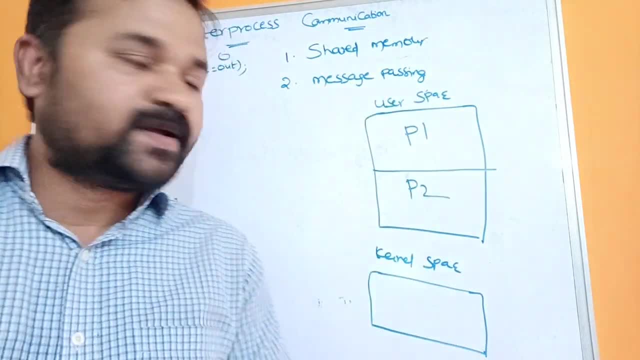 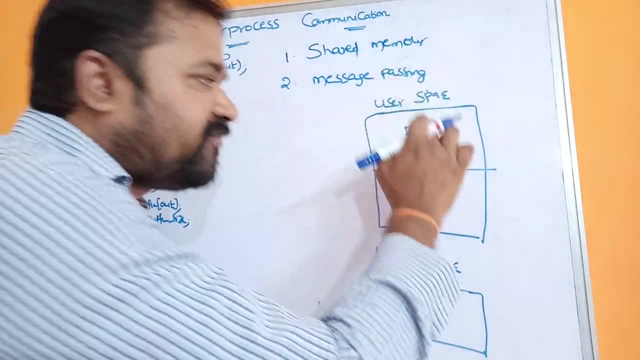 So here so how the message passing will be done. If- producer, if a process- P1 wants to send a message to P2, then first P1 wants to send a message to P2.. Then first P1 wants to send a message to P2.. 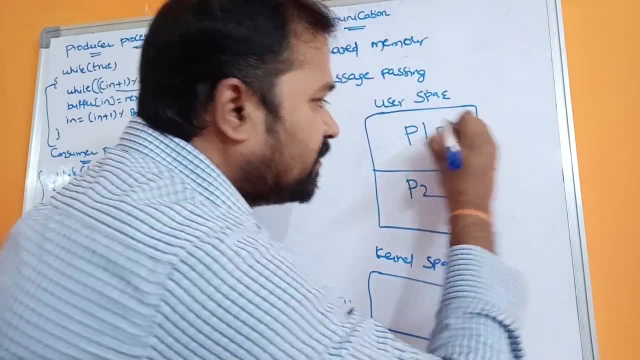 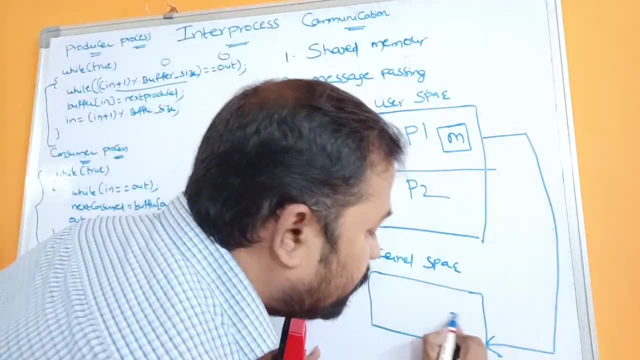 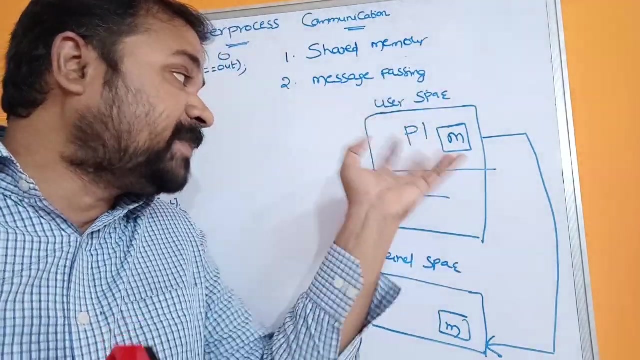 So first P1 has to send that message. Here M represents message. First P1 has to send that message to the kernel. So in kernel that message will be stored. Next if P2 wants to receive any message from the P1,. 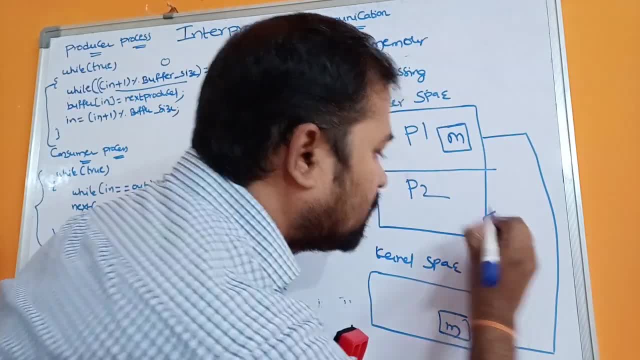 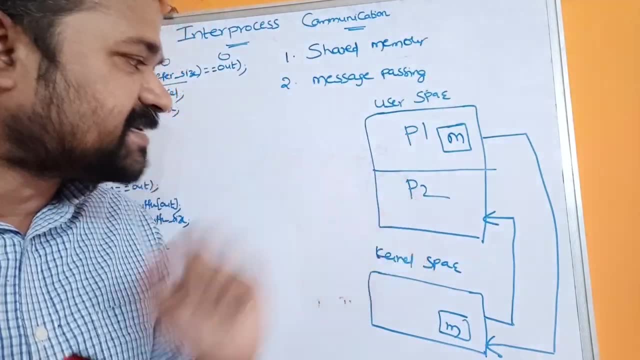 then it receives the message from the kernel. So here we are using what Kernel in order to pass the messages. So if P1 wants to send any message to the P2, then first P1 will send that message to the kernel. 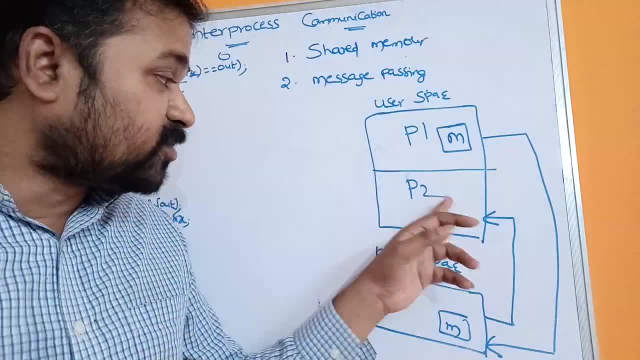 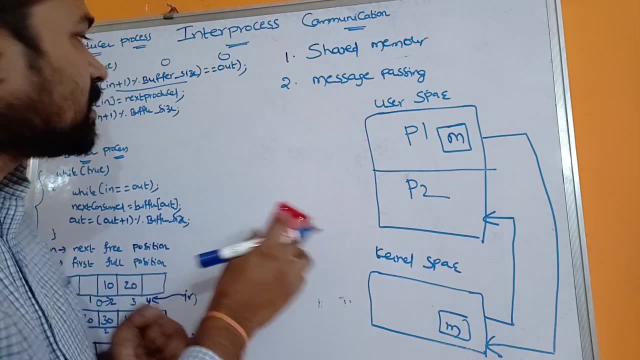 So in that kernel we have that message. So if a process P2 wants to receive the message from the P1, then it receives the message from P2.. Okay, Now let us consider some issues in message passing. So while implementing message passing, 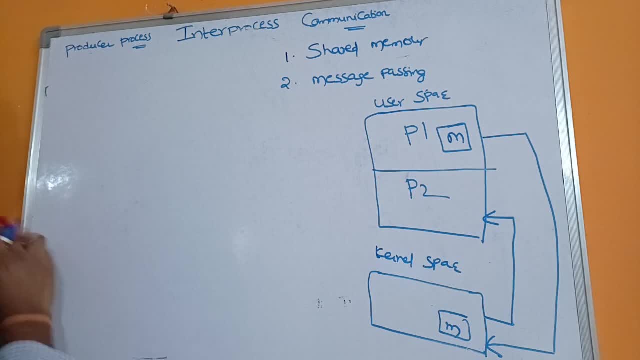 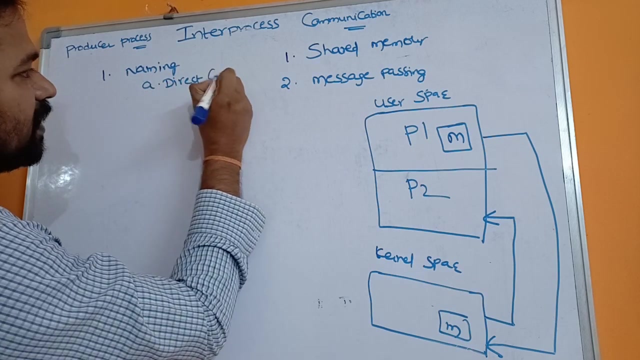 totally. we have to consider three issues. Let us see those three issues. The first issue is naming. So how sender will send the message And how receiver receives the message. So for that we have two approaches. We have direct communication as well as indirect communication. 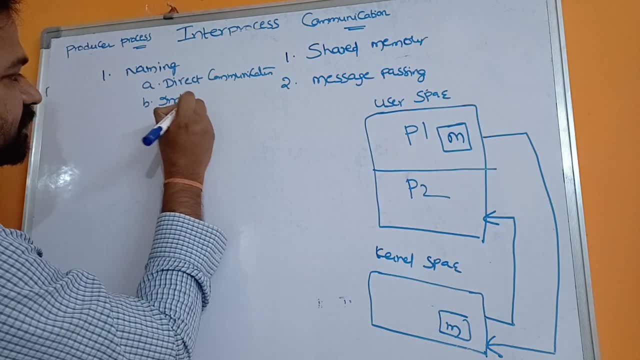 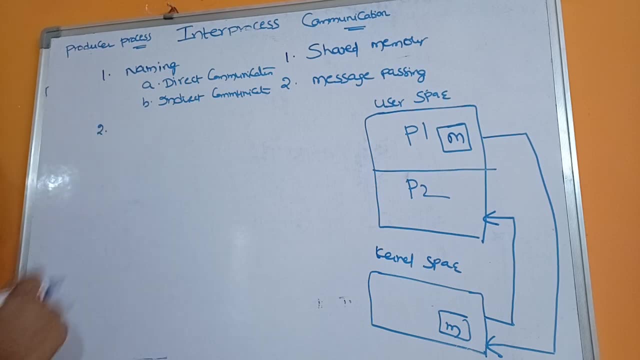 Direct communication as well as indirect communication. So by using these two approaches, one process can send message to another process And the second one is synchronization. So how we will implement synchronization? So we have to consider this also, Because there should be some communication between 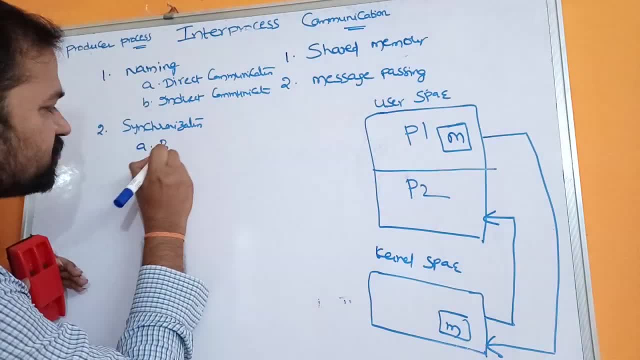 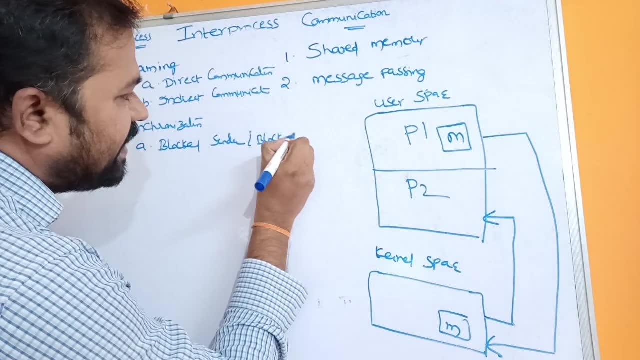 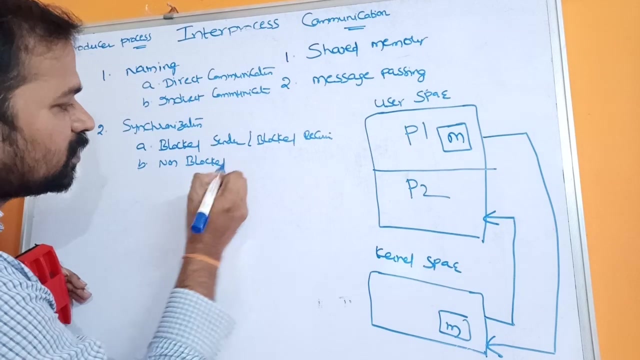 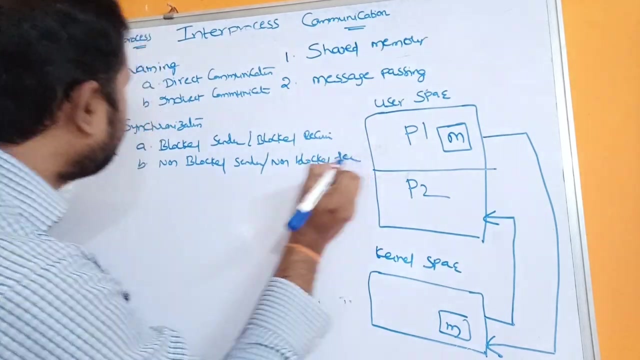 the sender and the receiver. So here we have two approaches. First one is blocked sender, blocked receiver, Blocked sender and blocked receiver, Whereas the second one is non-blocked sender, non-blocked sender and non-blocked receiver. So we have to consider about these two. 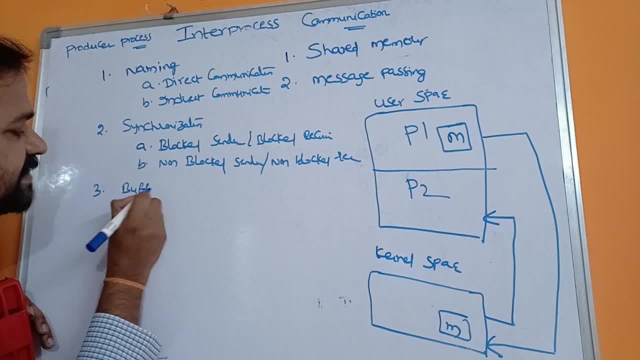 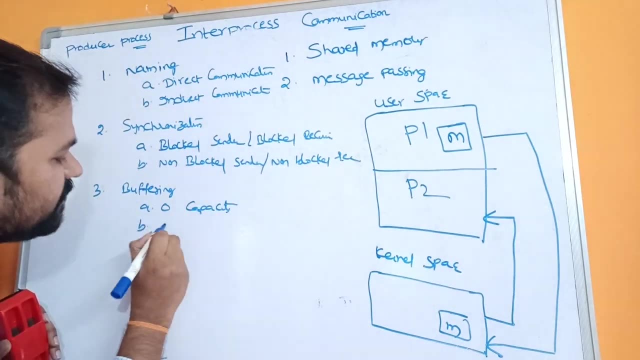 And the third one is buffering. So what is the size of the buffer? The size of the buffer may be zero capacity, Or the size of the buffer may be some finite capacity, Or the size of the buffer may be some infinite capacity. 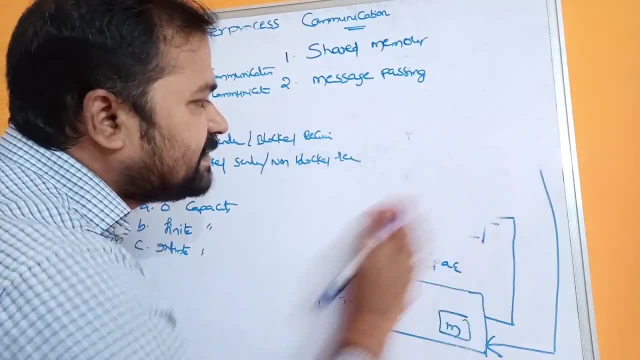 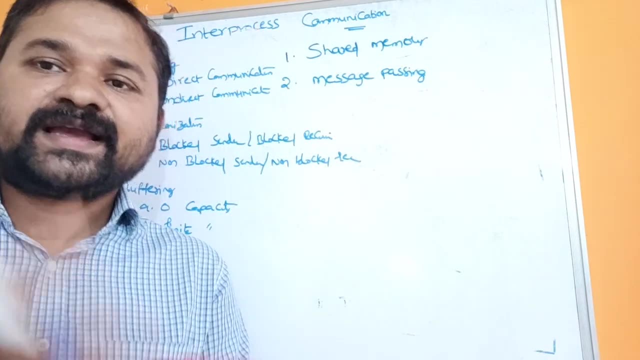 So we have to consider these three issues while implementing the message. So let us see the first one. What is the first one? Naming? Naming will specify how one process can send a message to the other process And how one process can receive the message. 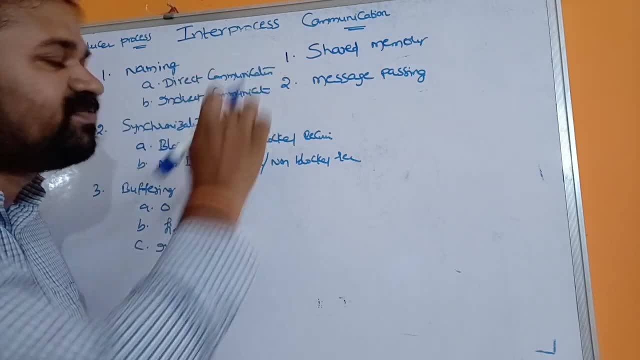 from the other process. Here we can implement the first one. Here we can implement the second one. Here we can implement the third one. Here we can implement this one with the help of two ways. First one is direct communication. Second one is indirect communication. 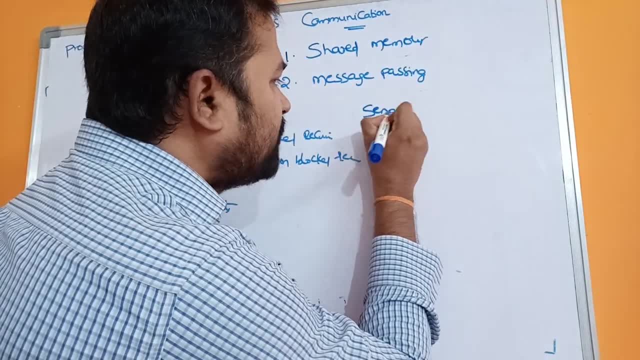 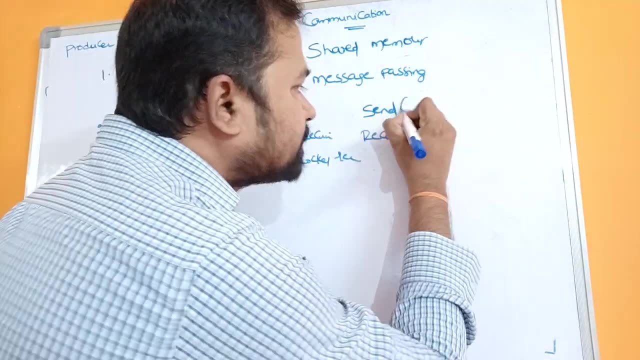 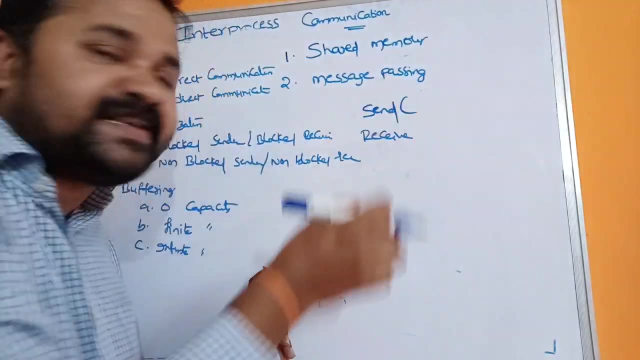 Here we use two operations. The first operation is sender operation- These are nothing but subsystem calls- And the second operation is receive operation. Direct communication means if the sender wants to send a message to the receiver, then it explicitly specifies the receiver process name. 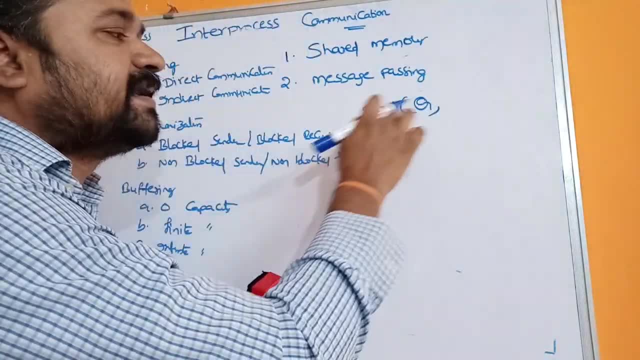 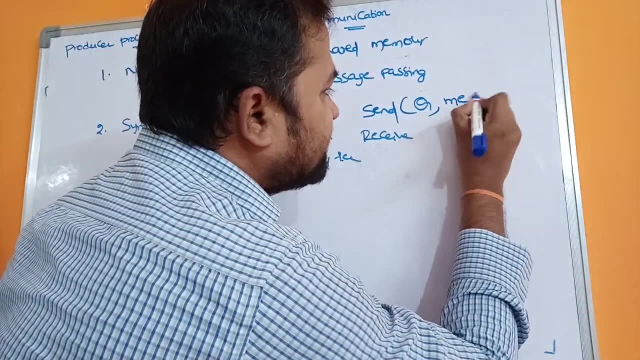 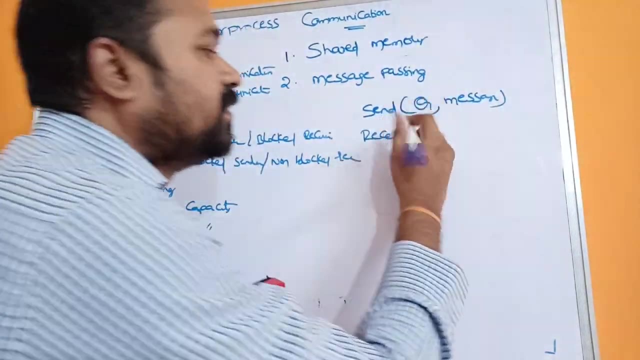 Let the receiver process name is Q, So the sender process explicitly specifies to which process that message has to be transmitted. So send Q message. So whenever this statement is executed, then this message will be sent to process Q. So likewise in direct communication. 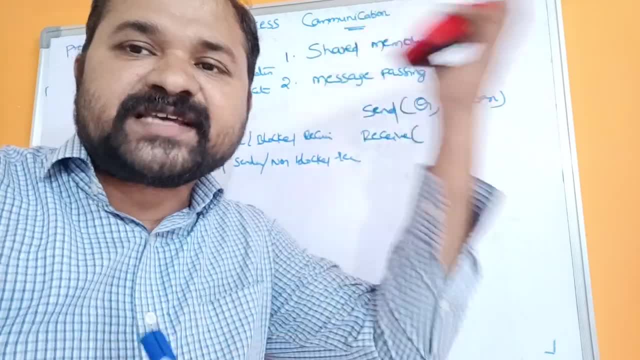 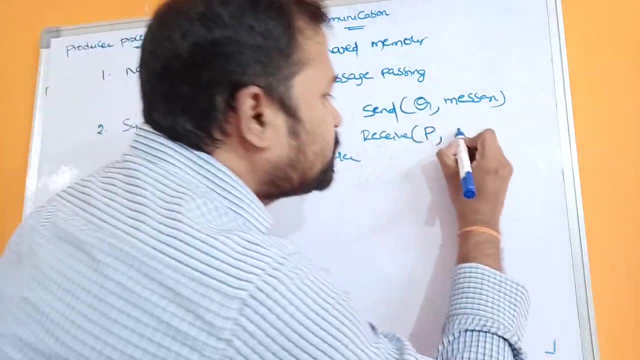 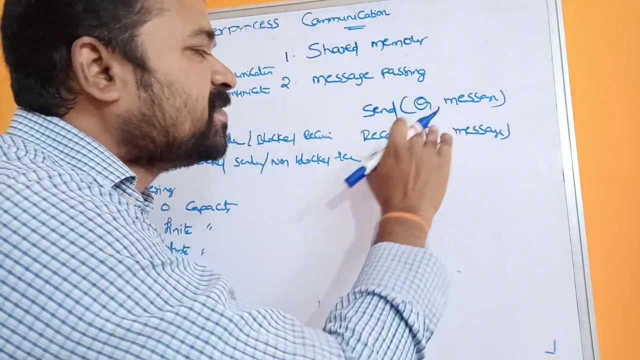 if receiver process wants to receive a message from the another process, then it has to be explicitly specifies from which process it has to get the message. So receive P message. So it specifies that receives the message from process P. So this is called as direct communication. 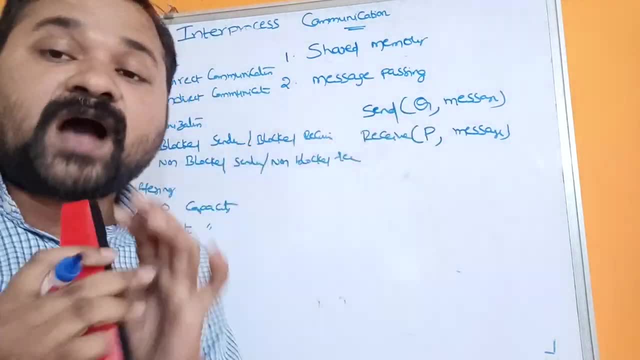 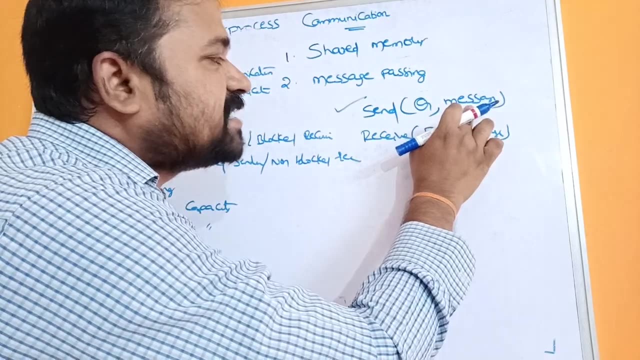 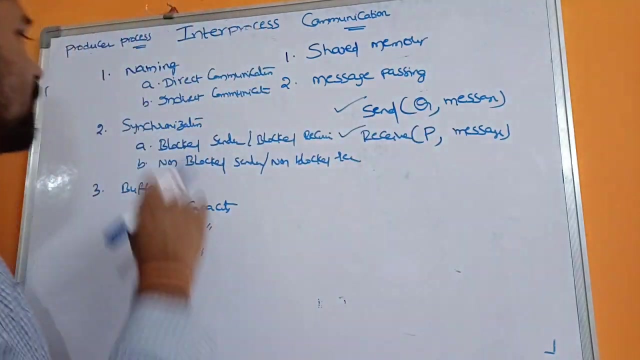 Direct communication means in the system call only explicitly. we have to specify the process name. So this statement specifies that: send the message to process Q. This statement specifies that receive the message from process P. Now let us see about indirect communication. 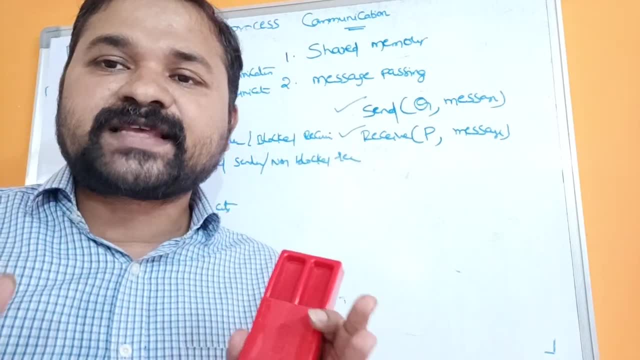 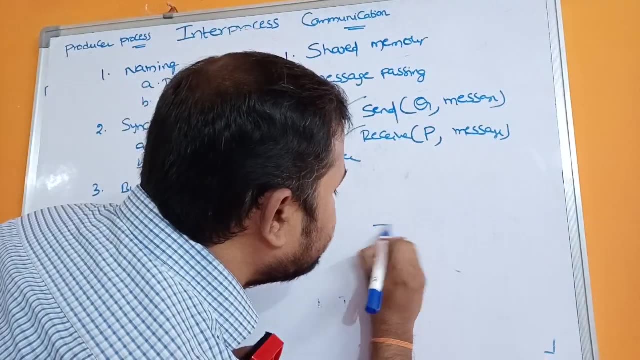 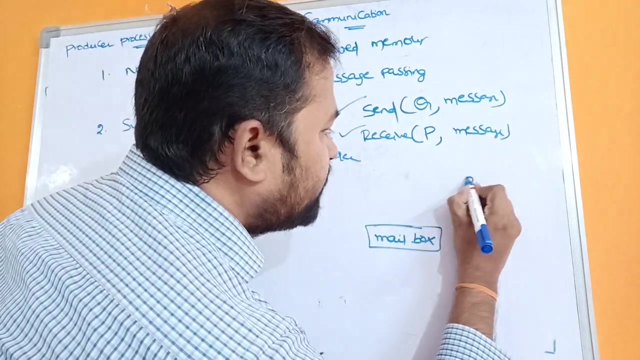 Indirect communication means the processes cannot receive and the processes cannot communicate directly. Instead, the processes uses a mediator. That mediator is called as mailbox here. That mediator is called as mailbox here. Like we have two processes, Process P and process Q. 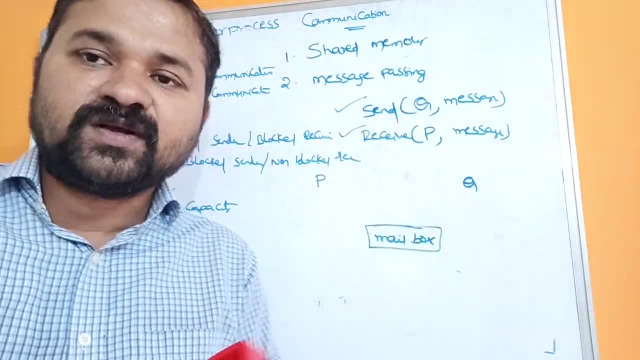 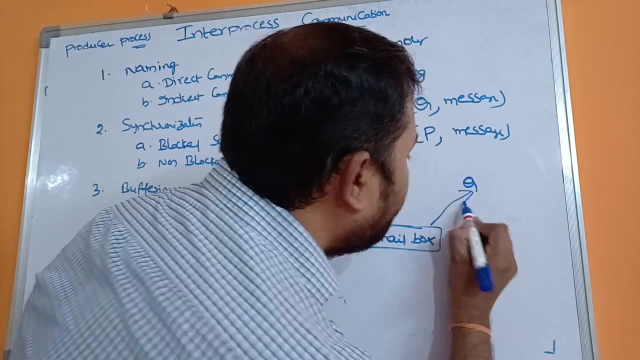 So if process P wants to send a message to process Q, So first the process has to send the message to mailbox. From the mailbox, process Q will receive the message. So where the mailbox will send Here the mailbox will receive in kernel only. 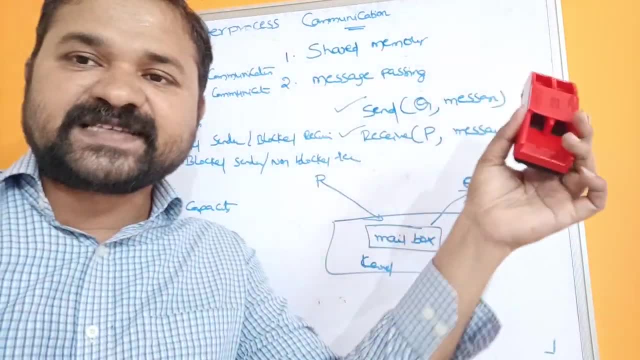 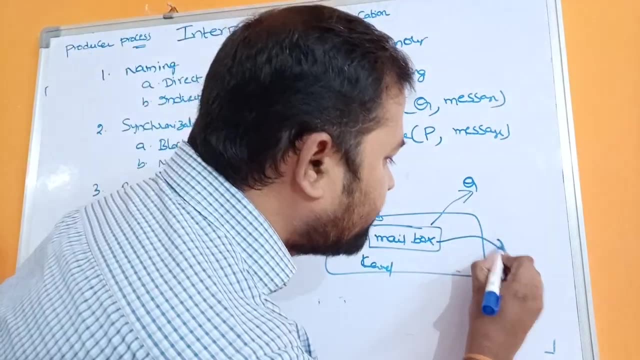 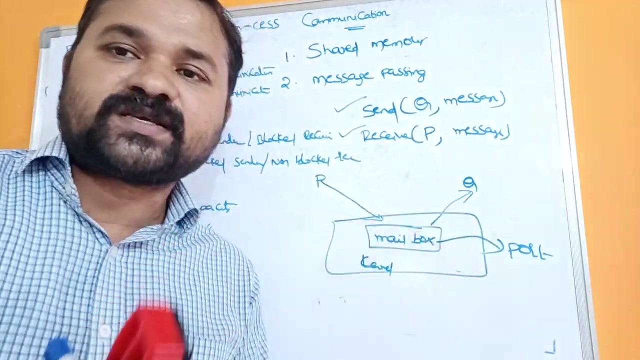 Kernel only. Why? Because already we have seen about what is message passing. That message will be stored in the kernel. Here, this mailbox, this is called as mailbox. This mailbox can also be called as a port. Here every mailbox has a separate identification number. 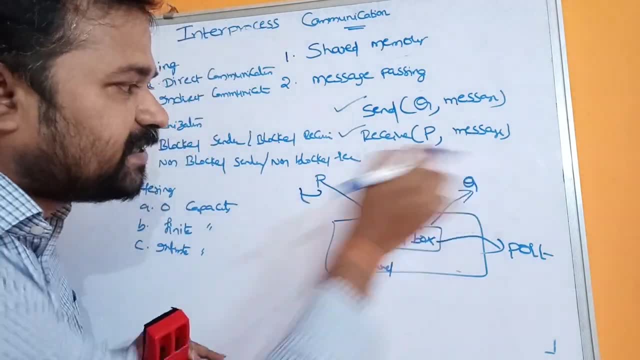 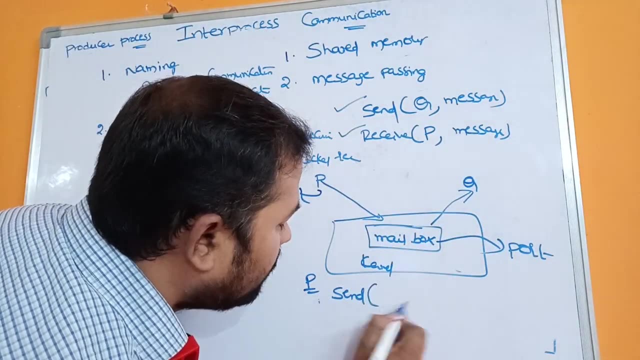 So if a sender wants to send a message to the- let us assume that closest P wants to send message to process Q- Then it executes a system call called send off. Let the ID of the mailbox is mailbox, So mailbox comma message. 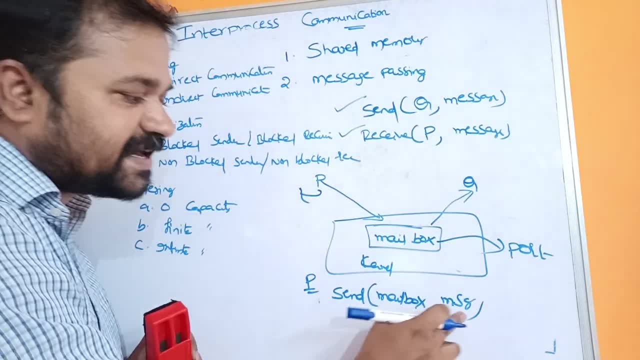 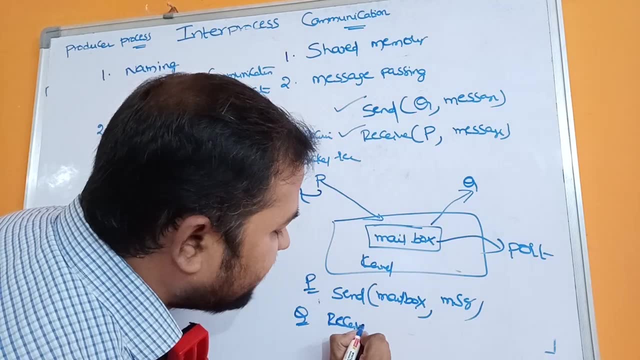 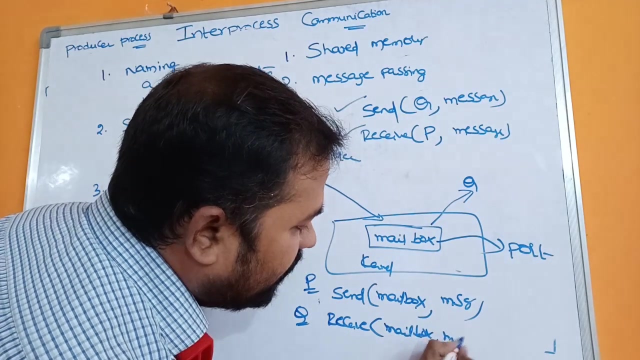 So whenever this statement is executed by process P, then the corresponding message will be sent to the mailbox. Now what the receiver will do? Receiver executes a system called receive off, Receive off mailbox comma message. So whenever process Q executes, 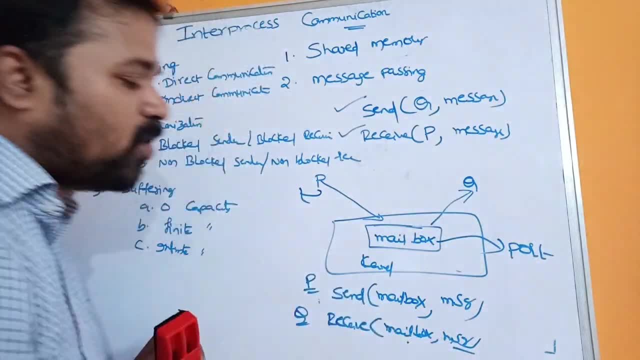 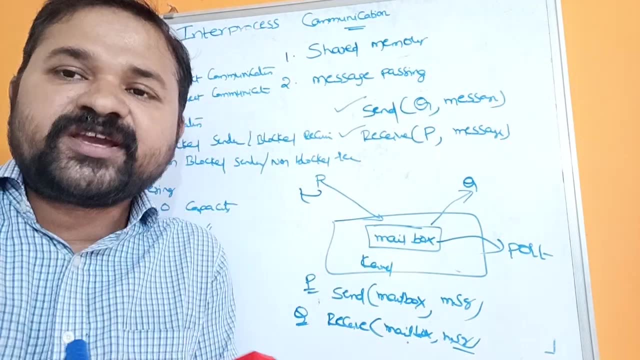 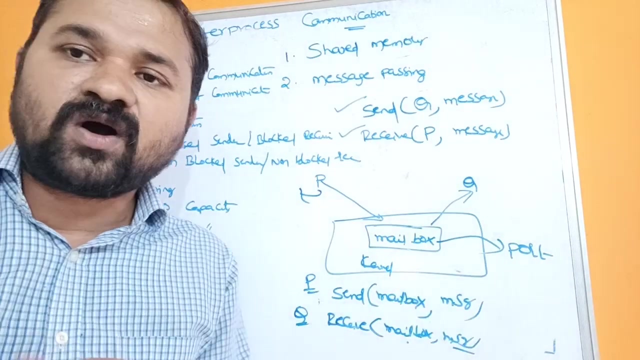 this system call, then it receives the message from the mailbox. So this is called as indirect communication. Indirect communication means the sender and the receiver will communicate with a separate mediator, a separate translator. So what is that mediator? Mailbox can also be called as a port. 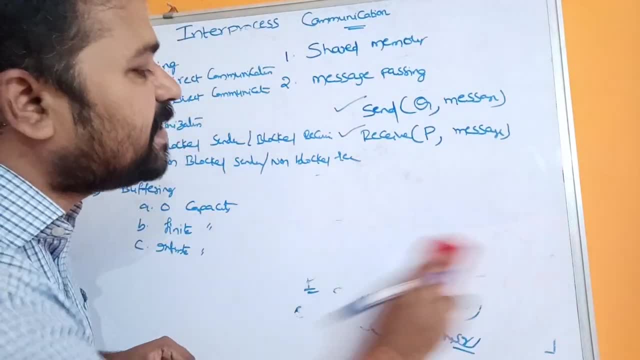 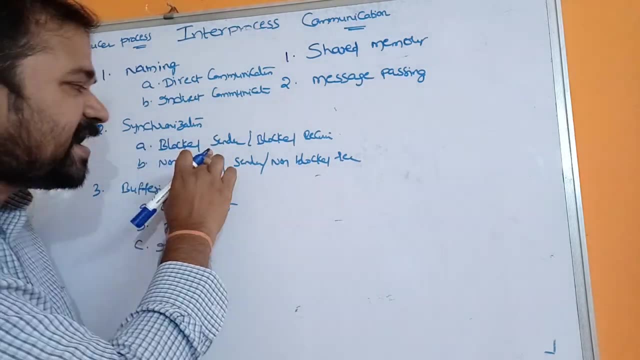 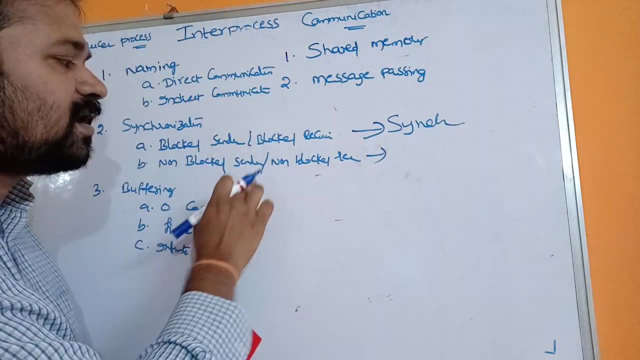 Now let us see about synchronization. So while implementing message passing, we have to take care about the synchronization also. Here we have blocker sender, blocker receiver. This will maintains synchronization, Whereas non-blocker sender or non-blocker receiver is asynchronous mechanism. 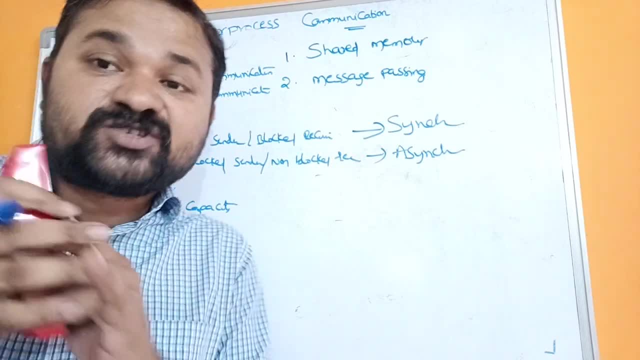 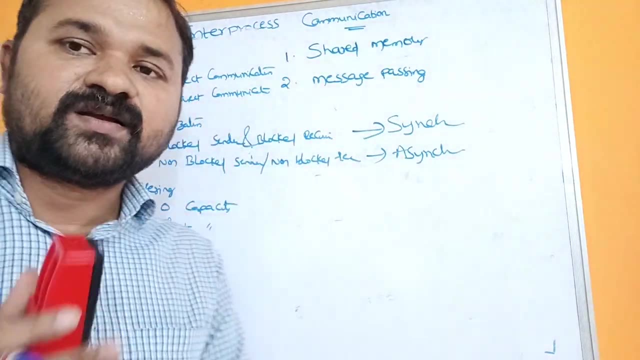 Here. if you want to maintain a synchronous mechanism, then we should have to implement blocker sender or blocker receiver, Blocker sender and blocker receiver. So what is blocker sender? Blocker sender means sender sends the message After sending the message. 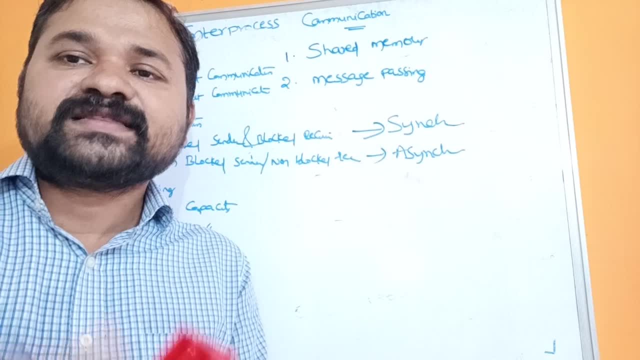 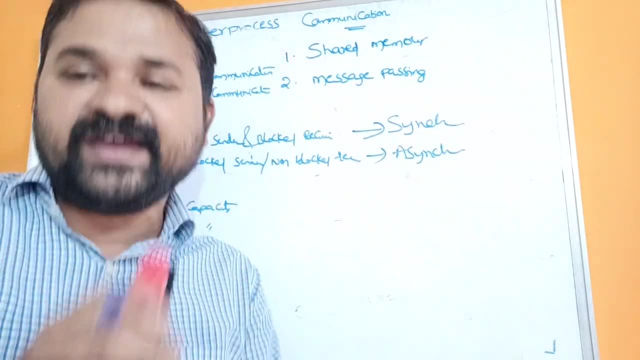 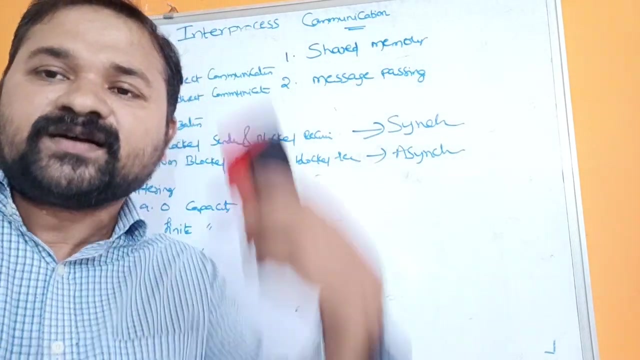 the sender process will be blocked until the receiver receives the message. If the receiver is busy with some other work, then the sender process has to wait until the receiver receives the message. So once the receiver receives the message, then only sender has to send some other message. 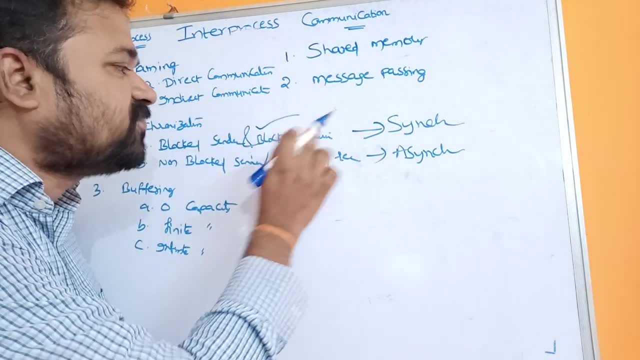 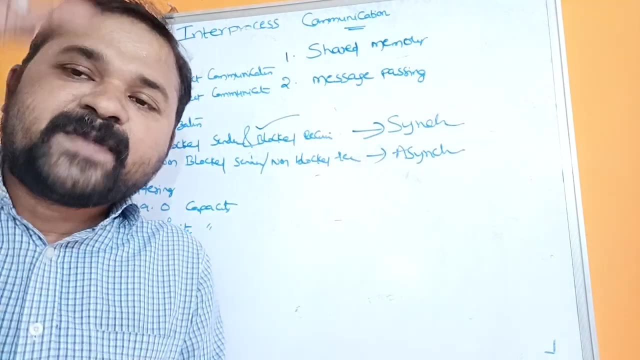 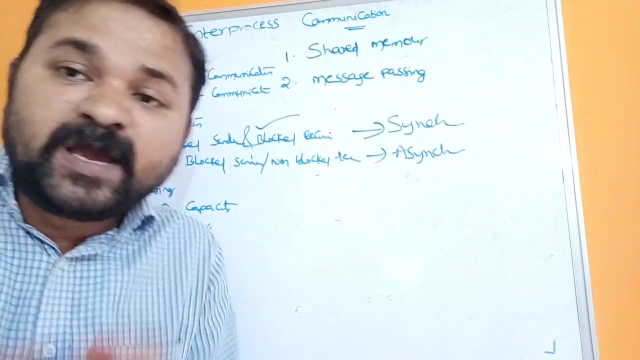 That is called as sender, blocker, blocker, sender. Whereas what is blocker receiver? Blocker receiver means the receiver process must be blocked until that message will be received by the sender. So what is blocker receiver? The receiver process will be blocked until that message will be received by the sender. 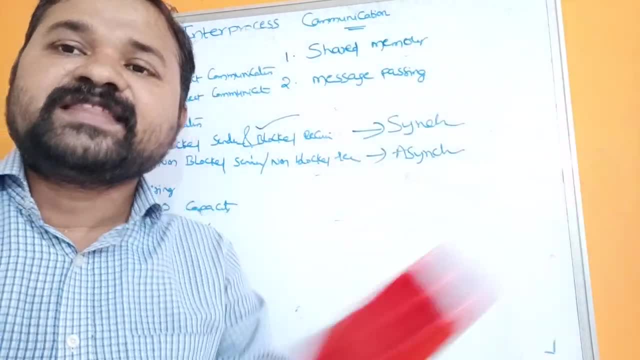 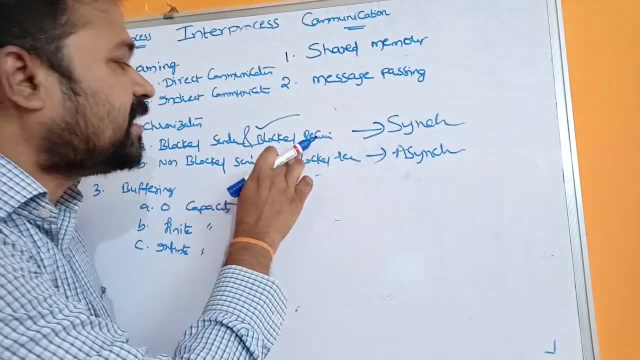 If the sender process is busy with some other work, then the receiver process has to wait until the sender receives the message. So if we implement blocker sender and blocker receiver, then we can implement synchronization. And what is the next one? Non-blocker sender means: 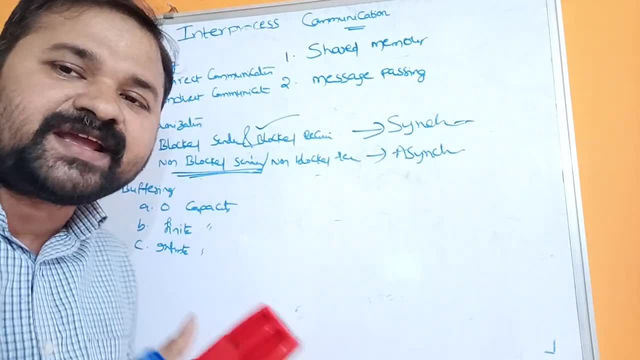 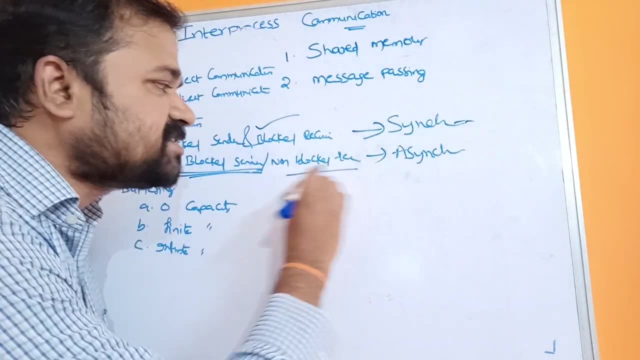 sender sends the message and after that it can continue with other work. It doesn't bother about whether that message is received by the receiver or not, Whereas what is non-blocker receiver? Non-blocker receiver means the receiver will receive its own work. 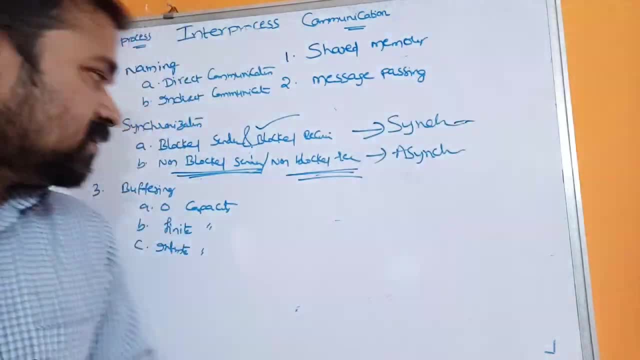 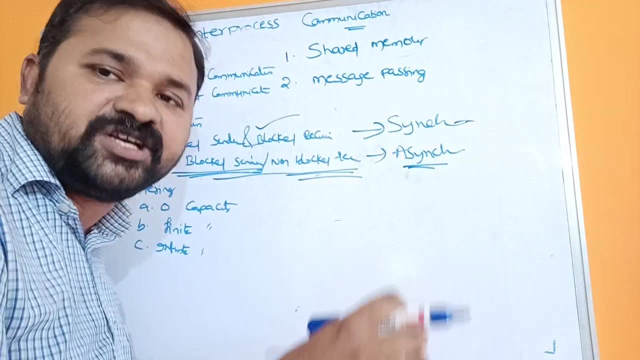 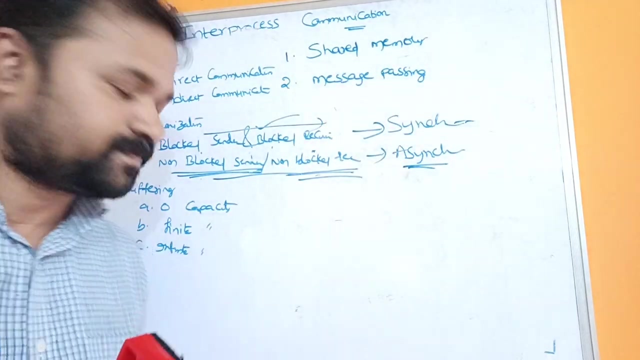 whether that message was received or not. So these two doesn't implements asynchronous. these two doesn't implement synchronization. So if we want to implement synchronization efficiently, then we have to implement this one blocker sender and blocker receiver. We have to implement message passing. 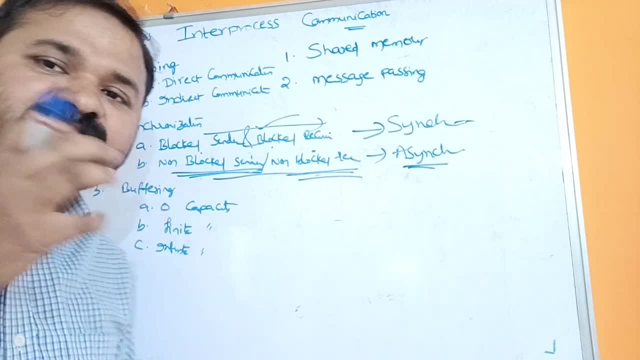 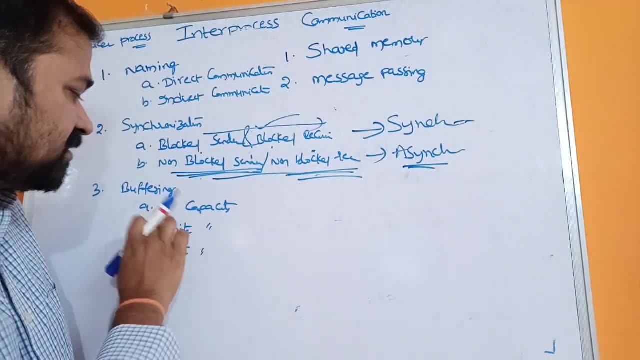 Now let's see the third one: buffering. So buffering means what is the size of the buffer? The buffer size may be either 0 capacity or finite capacity or infinite capacity. So 0 capacity means what? There is no buffer. 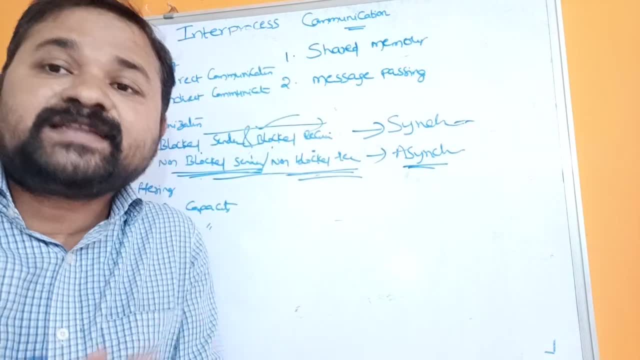 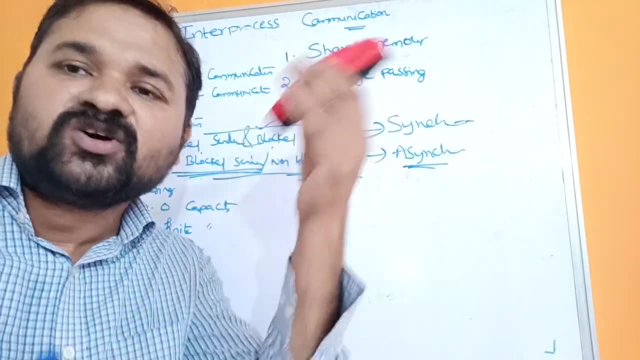 If there is no buffer, then if sender sends an item, then the sender has to wait until the receiver receives that item, Because there is no buffer here. so it is not possible to store that item in the buffer. So once the sender sends the item, 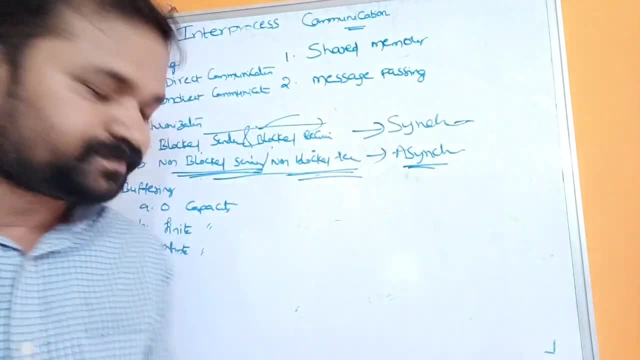 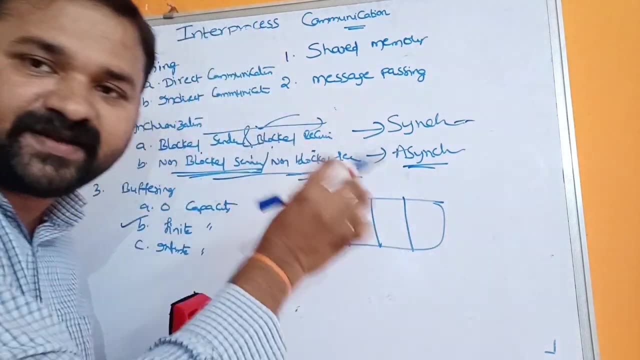 then it has to wait until the receiver receives the item. And the second one is finite capacity. So finite capacity means the size of the buffer is limited, finite. Let the size of the buffer is 5.. So this is nothing but finite buffer. 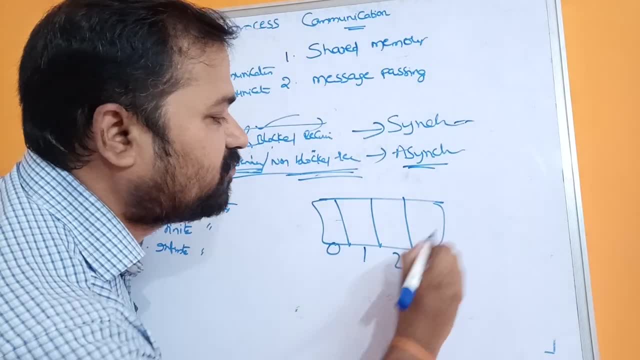 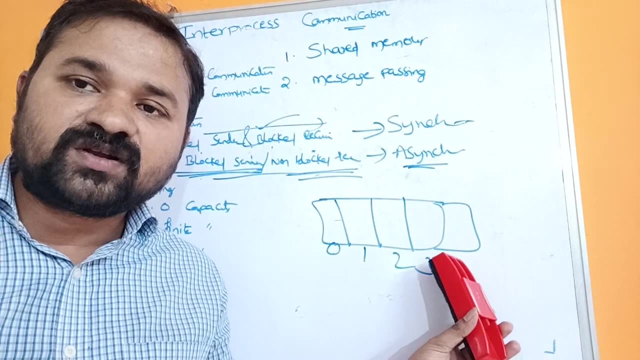 Let the size of the buffer is 5.. So then we can have 5 items landed, from 0 to 4.. So what is the problem here? Let the buffer is full. Let the buffer is full, Then the sender has to wait. 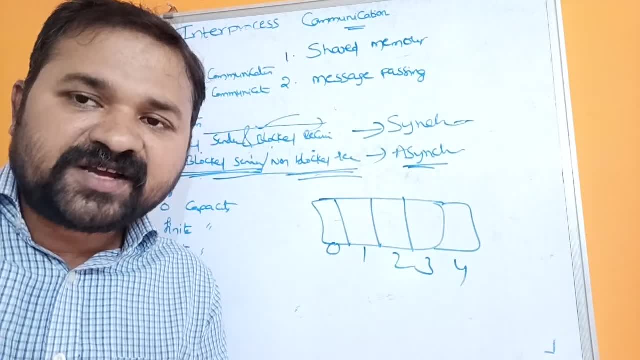 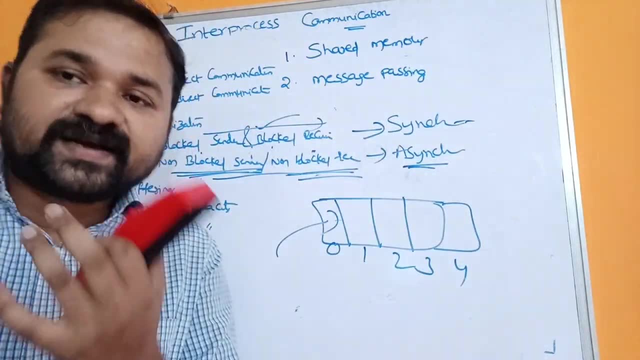 until the receiver consumes the item. If the receiver consumes the item, then only sender can put some other item in the buffer. So after the receiver receives the item, then sender puts some more item in the buffer, Suppose if the buffer is not full. 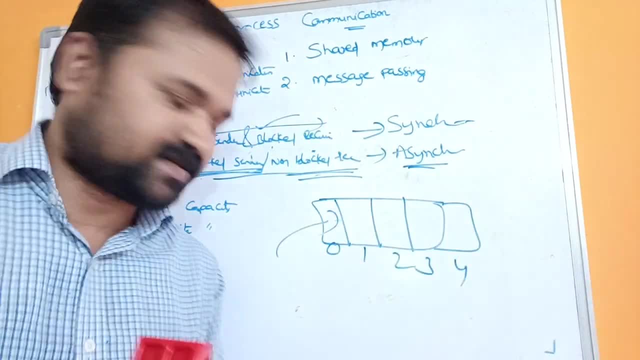 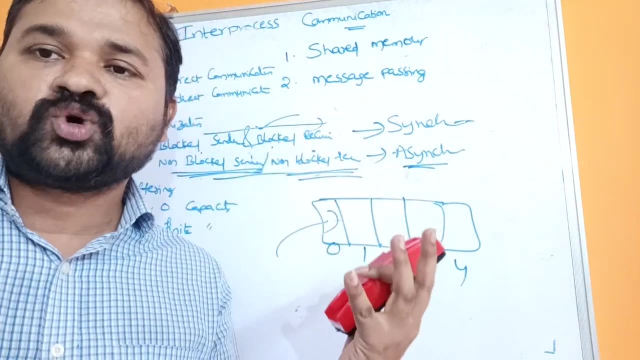 then there is no problem. Sender places some items in the buffer. The last one is infinite capacity. Infinite capacity means the buffer size is infinite, So there is no need to wait by the sender. So sender can put any number of items in the buffer. 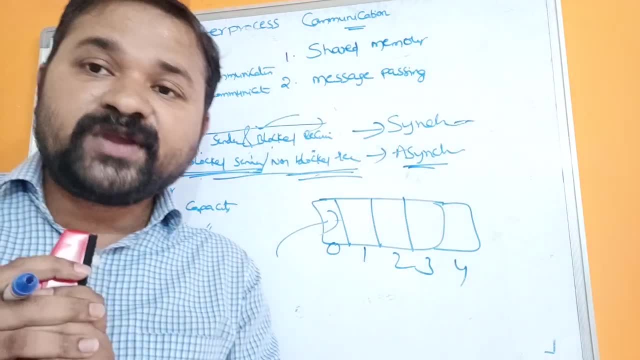 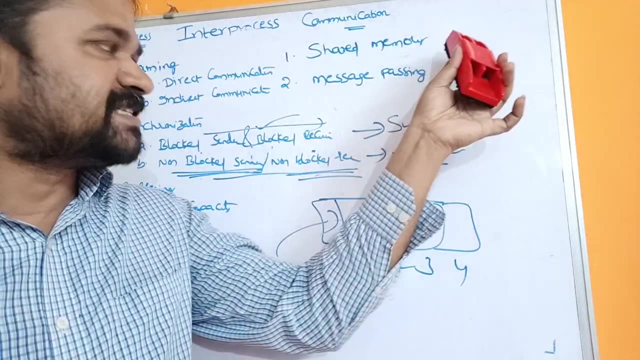 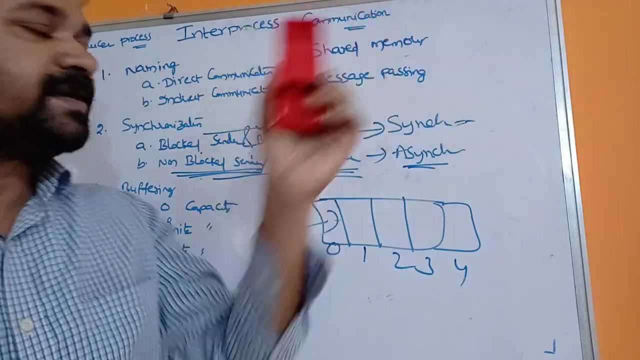 So this is about message passing. So, in order to implement inter-process communication, we can make use of either shared memory as well as message passing systems. In the modern days, all the operating systems are using these two mechanisms in order to implement inter-process communication.